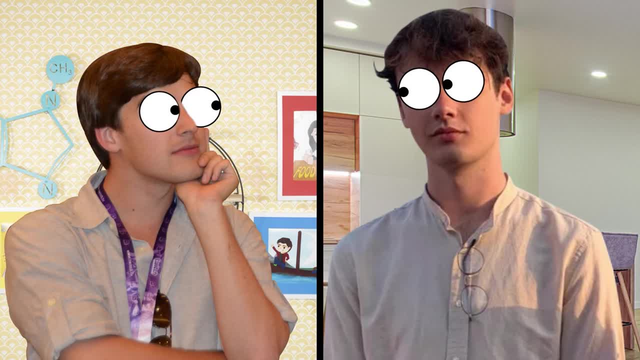 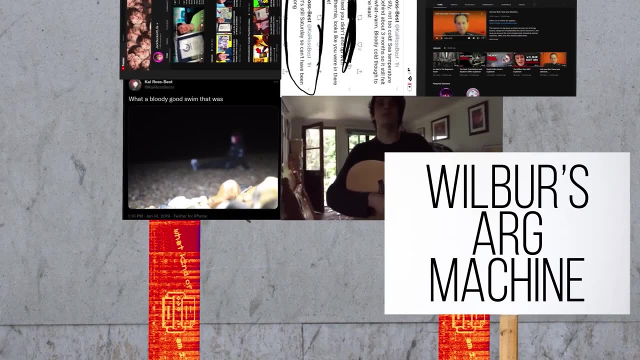 He told me that, while it is technically solvable, he would actively discourage me, as well as anyone else, from attempting to solve it. He reiterated this a bunch during our call, claiming that the ARG was poorly constructed, with puzzles that were accidentally made too hard. 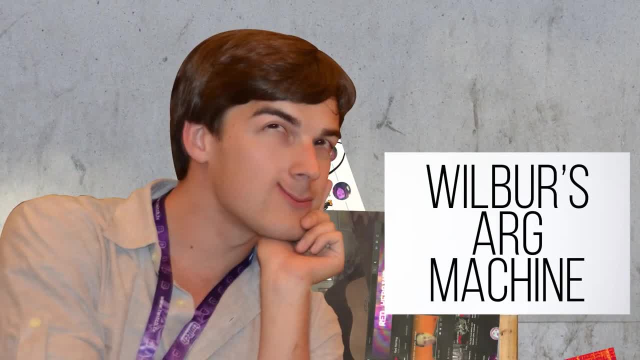 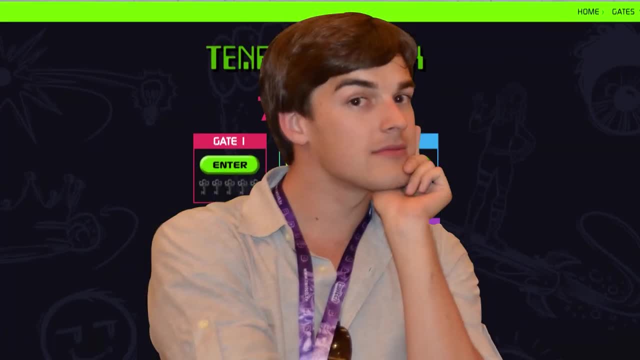 And not hard in the good way of wow, that was really challenging to figure out, but rather hard in the frustrating oh, how could I have ever known to do that sort of way? And I get it As someone who's done his own ARGs a few times. 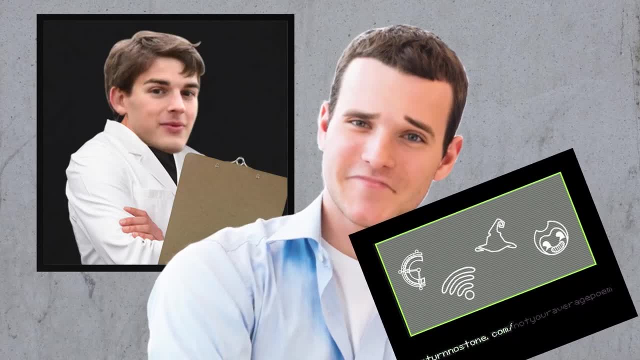 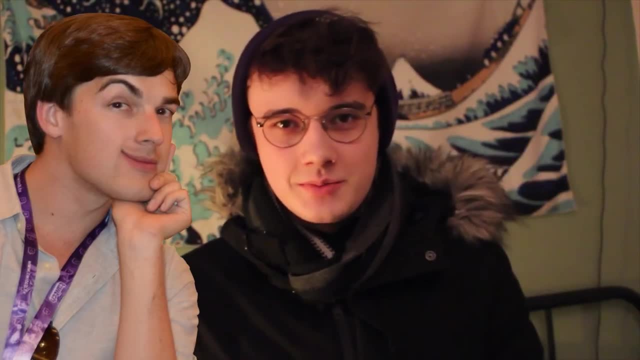 finding the right level of difficulty is really tough. People take clues and directions that you could have never suspected And I gotta say it is awesome that Wilbur acknowledges and admits all of his first-timer faults. I respect that a lot. I also choose to completely ignore him. 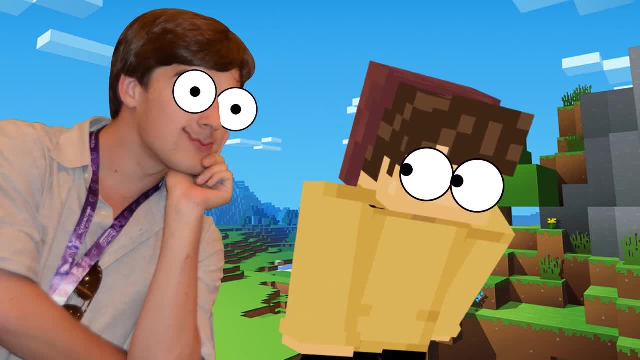 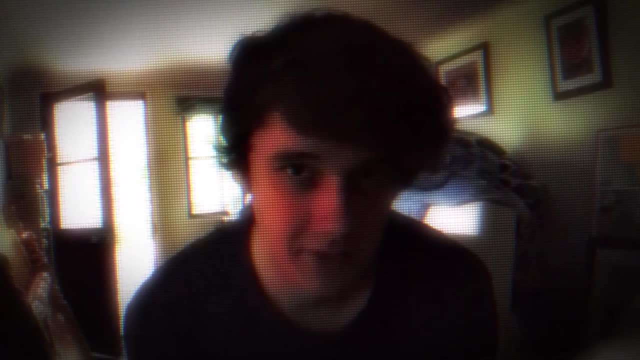 Sorry, Wilbur, you're a good dude, but you know that I couldn't leave this ARG incomplete. And I gotta say I think I solved it. I think I have some solid answers to the ARG's biggest lingering questions. But to understand how? 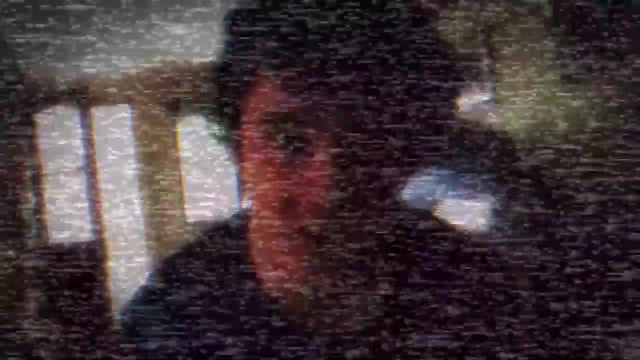 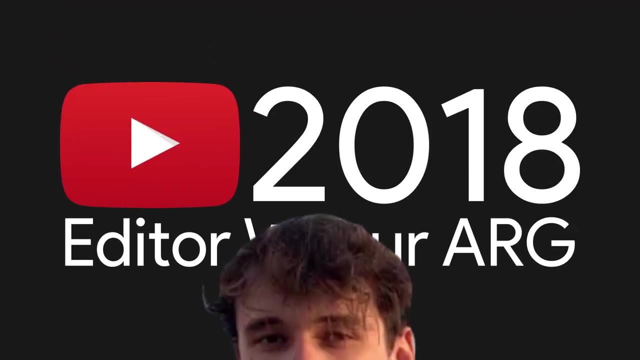 you first have to understand what exactly this thing was and what made it so hard. The editor Wilbur ARG officially kicked off back in December of 2018, but Wilbur had actually been seeding the idea of doing an ARG for nearly a year before that. 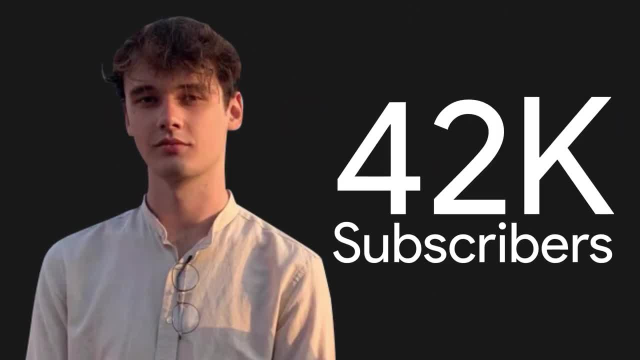 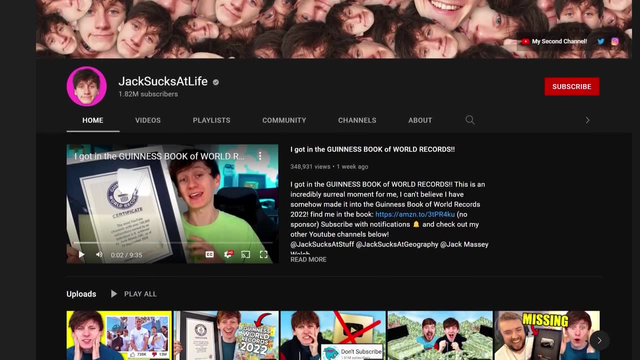 Despite having a channel of his own with over 42,000 subscribers. at the time, the ARG wasn't actually started there. Instead, the whole thing kicked off when another channel, JackSucksAtLife, uploaded the ominously titled: I let a random guy edit this video. 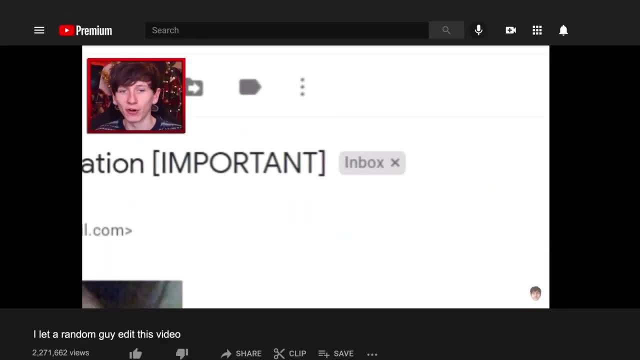 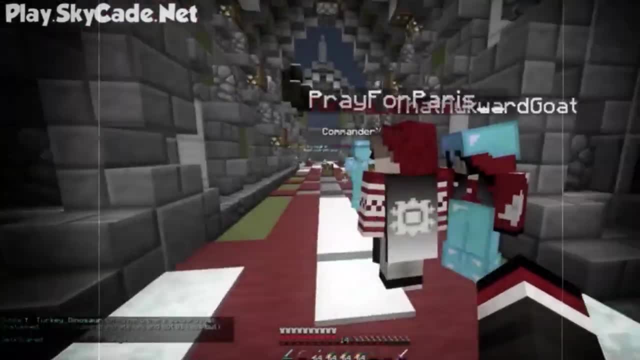 Six days ago I get this email titled new editor application important And I think: well, I'm not looking for a new editor. Nowadays, Jack collects YouTube play buttons, but back then he was predominantly a Minecrafter. Also on that note, Jack. 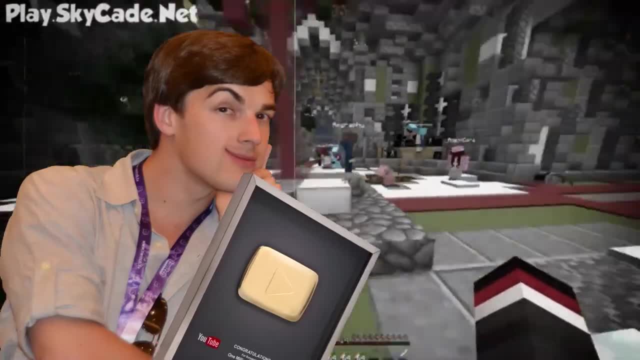 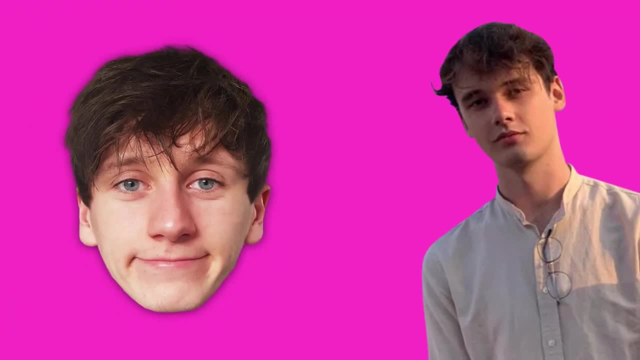 I have the one version of the gold play button that you don't have, As far as I know. it's the only thing missing from your collection. I'm just saying let's talk. According to Jack, he was contacted by a person named Wilbur, looking to apply for a job as editor. 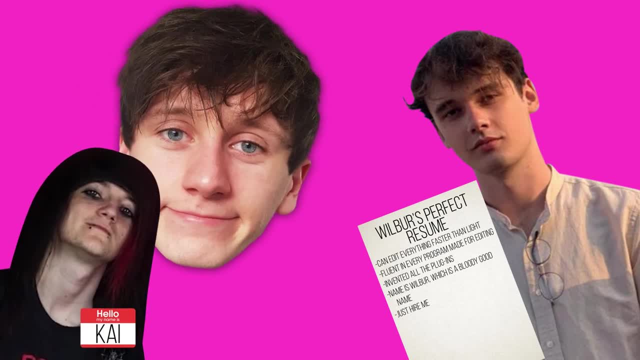 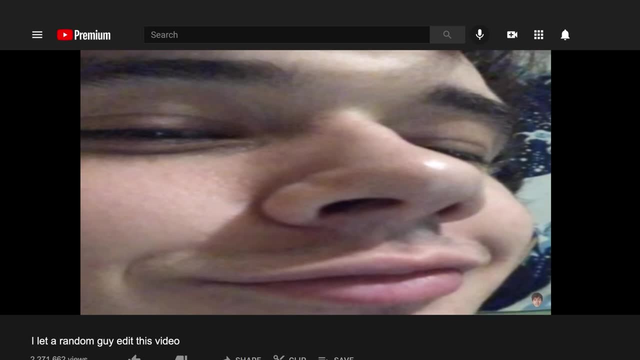 which immediately is weird, considering Jack already had an editor. But things get weirder once he opens the email, which begins with a giant image of Wilbur and a rant against Jack's current editor. Kai, Now I know what you're thinking. 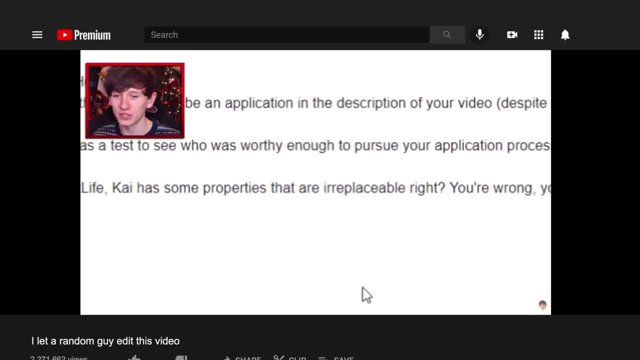 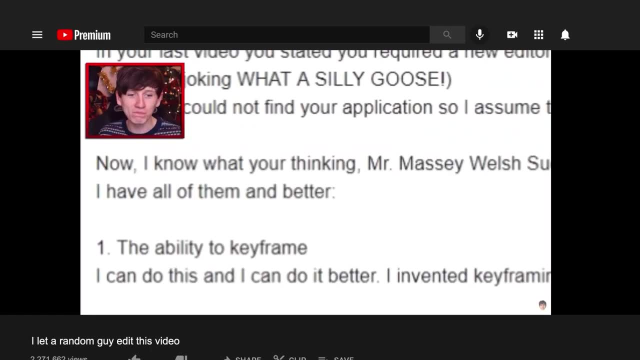 Mr Massey, Welsh sucks at life. Kai has some properties that are irreplaceable. right, You're wrong, You idiot. I have all of them, and better What? Who? Wilbur, Wilbur then out of nowhere. 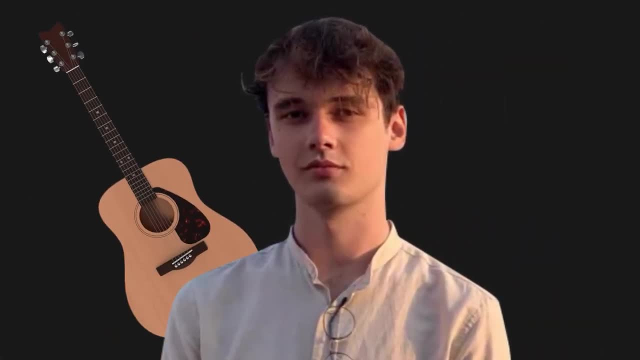 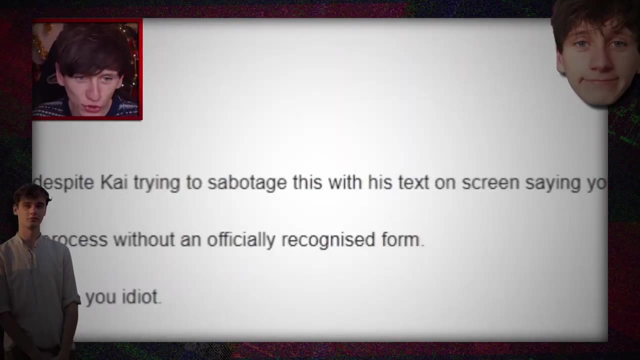 claims to have invented two of the six strings found on a guitar, as well as the editing tool of keyframing, which means, I guess, I owe the dude a fortune in royalties. Despite all of these red flags, Jack decides to let go. 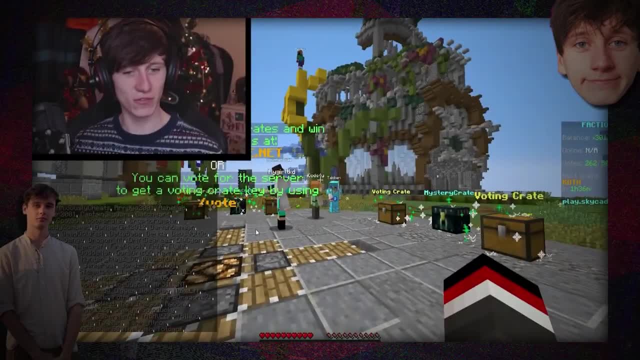 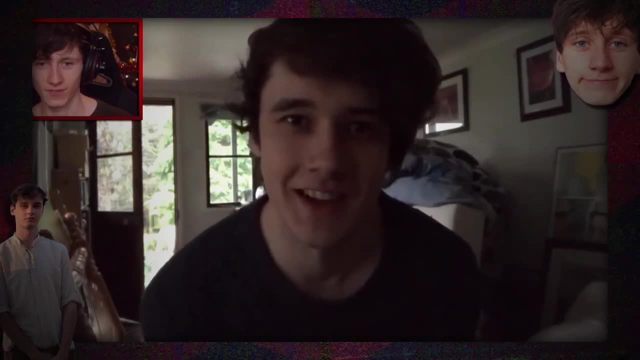 let Wilbur go ahead and edit part of the video and things start out pretty normally, At least until the middle, when we switch to a video of Wilbur completely taking over and introducing himself to Jack's audience, appearing in a decrepit old house in the middle of nowhere. 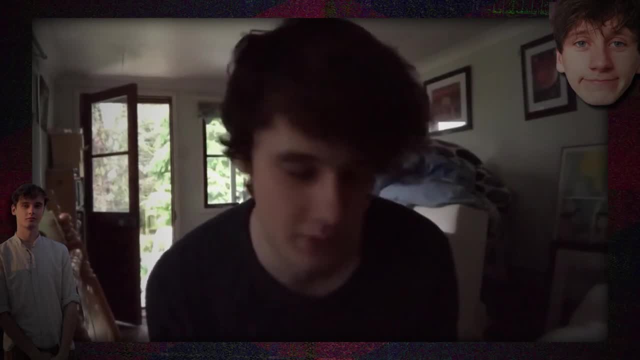 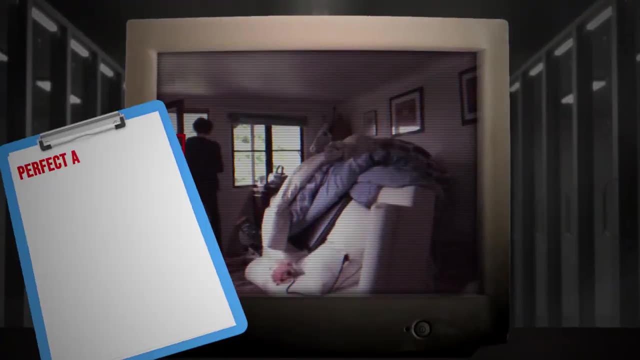 where no one can find you saying that there are people chasing him and that he's suffering from frostbite. He begins to play a song and then there's a loud thud heard from off screen and he runs away. It is pretty much the perfect first ARG video. 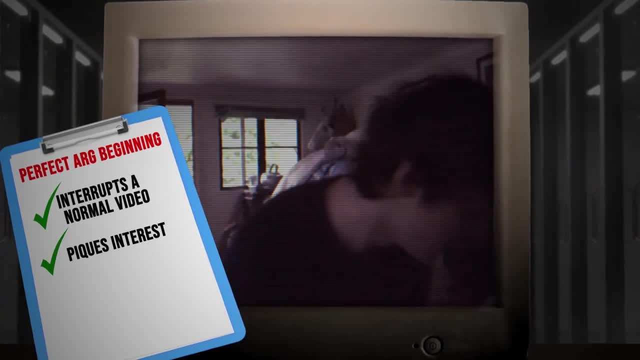 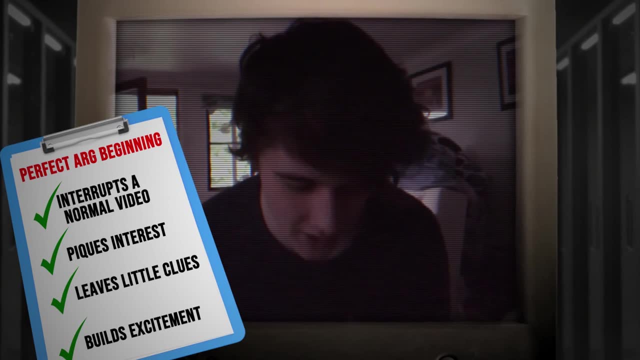 You interrupt a normal piece of content, you pique their interest with a couple of mysteries, leave little clues that don't make a whole lot of sense on their own and build excitement for the next video, A next video that would happen a mere four days later. 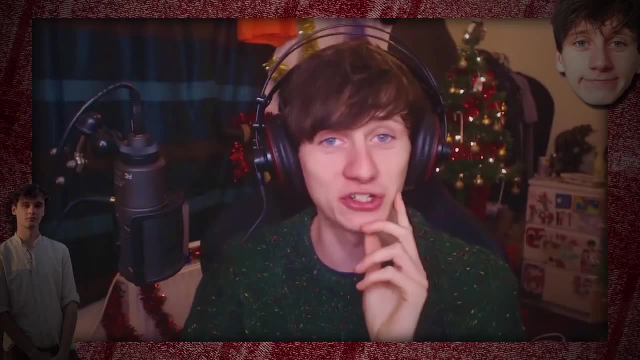 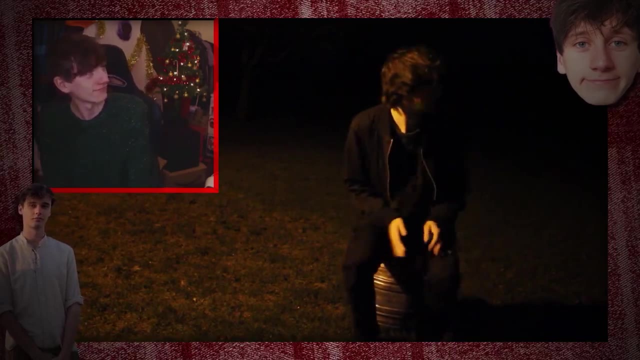 The second video entitled. I Let Him Edit Another Video. This Is What He Sent Me Back is pretty normal until we get to the end. Jack asks Wilbur to play a song while he sways in the corner, but all we see is Wilbur sitting on a keg. 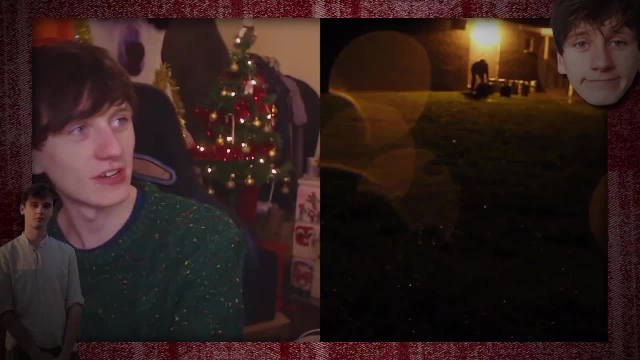 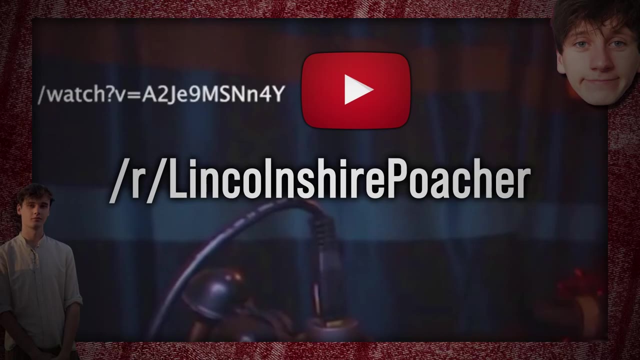 I haven't got a song for you, Wilbur, thank you. After that, things continue on until the very end where, in the top left-hand corner, we're given a U-turn, A URL to an unlisted video called Our Lincolnshire Poacher. 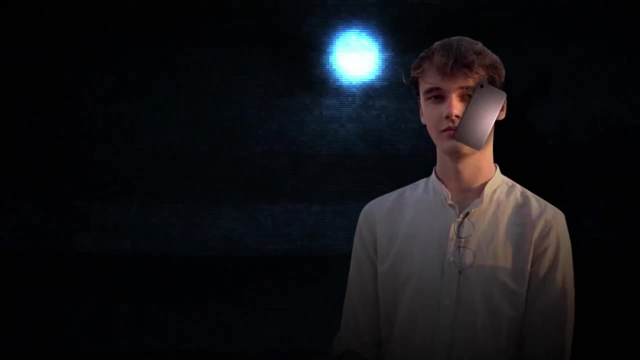 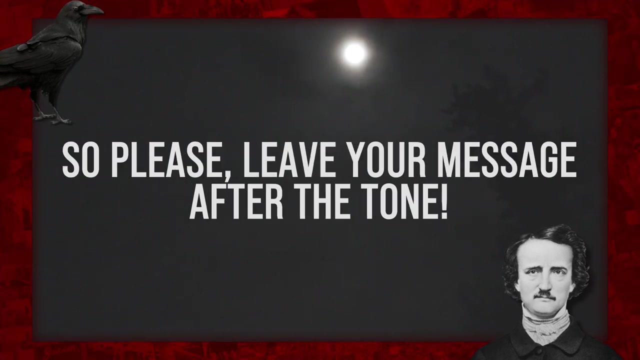 itself a reference to a subreddit. In this video, we hear Wilbur leave a voicemail for someone reciting the poem The Raven by Edgar Allan Poe. Hello, your call cannot be taken at the moment, so please leave your message after the tone. 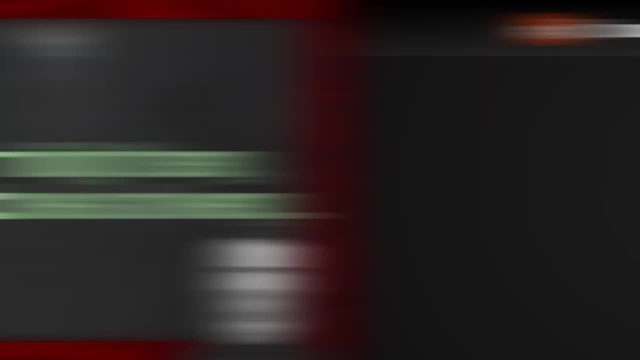 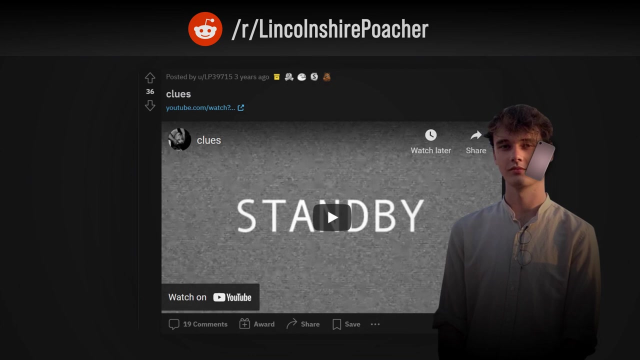 Once upon a midnight dreary while I pondered, weak and weary, If you go over to the subreddit, you're greeted with yet another video called Clues. This again has Wilbur leaving a voicemail and reading yet another Edgar Allan Poe story. 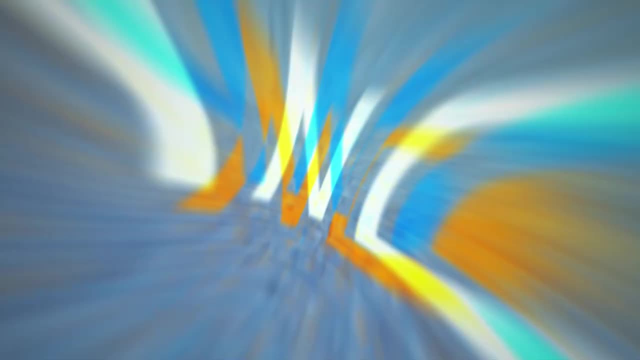 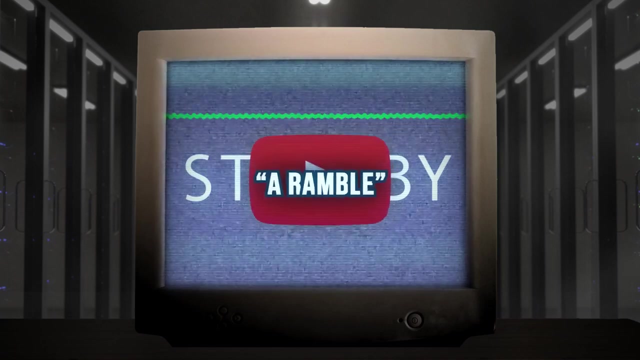 but this time the short story, The Cask of Amontillado. Listen until the very end, though, and you hear Morse code playing. It's a reversed base-64 code, leading to yet another YouTube-unlisted video entitled A Ramble. 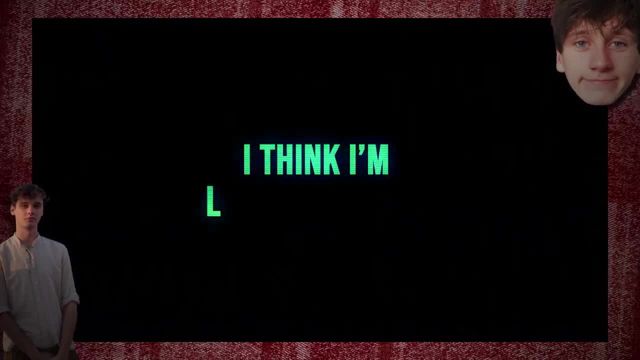 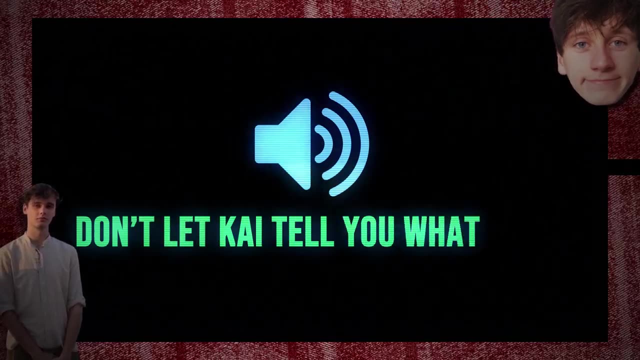 If you're watching this, Jack Massey well, sucks at life. I think I'm losing my mind anyway. so At the end of this one there's yet another Morse code, this time translating to: Don't Let Kai Tell You What I Did. 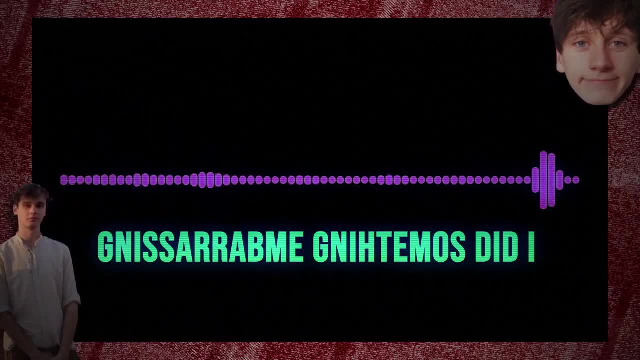 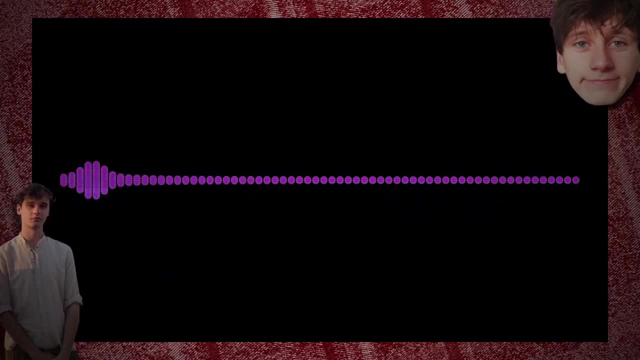 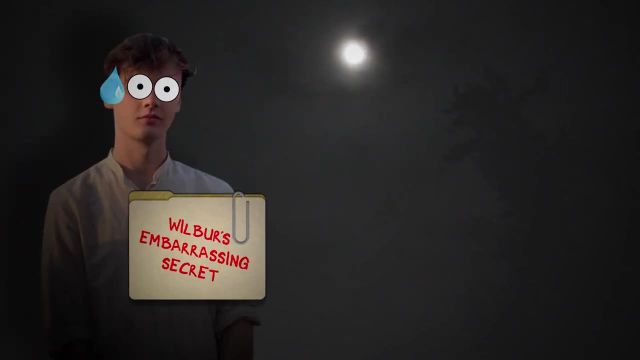 This ties in with a phrase repeated by a synthetic voice: I did something embarrassing. I did something embarrassing. Now we're starting to piece together elements of a story. Wilbur is embarrassed about something he did, something that has perhaps forced him to live on the run. 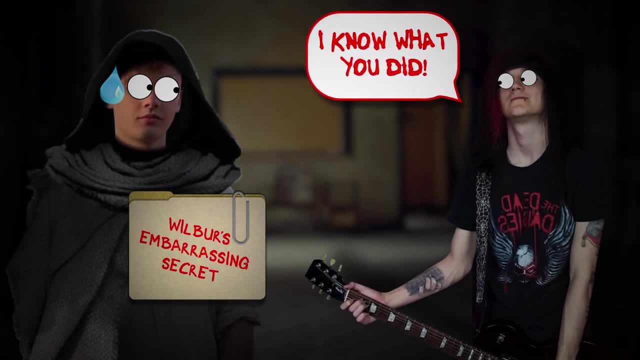 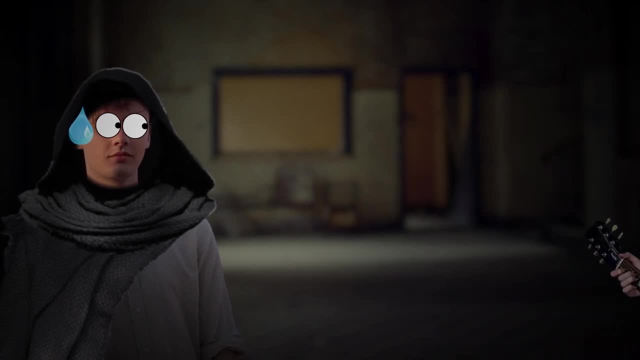 Apparently, Kai also witnessed this event, or else Wilbur accidentally let what he did slip to Kai and is now afraid of what might happen if word gets out. hence him wanting Kai removed from the position of editor, a position where he has a voice and could likely spill the beans. 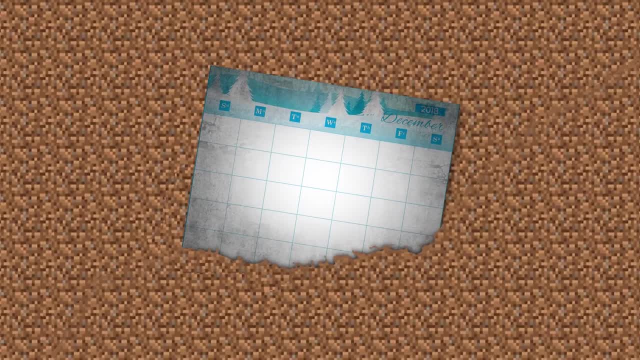 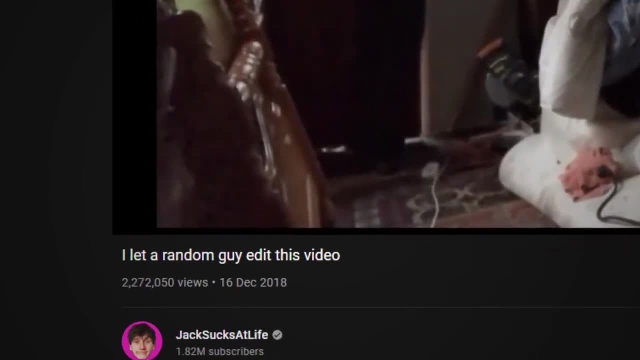 Digging deeper, though, we can actually pinpoint the window of when the event happened and when Wilbur's feelings towards Kai shifted. The first video of the ARG was in December of 2018.. However, if you check Wilbur's Twitter from a few months earlier, 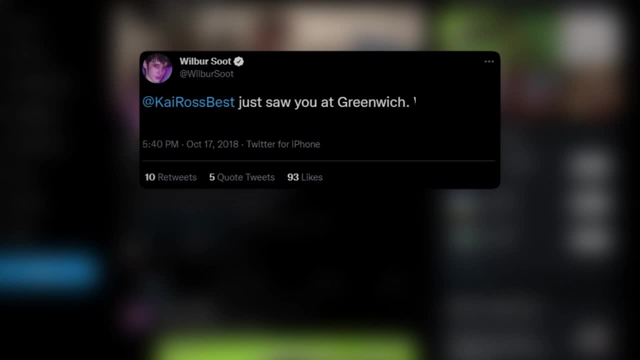 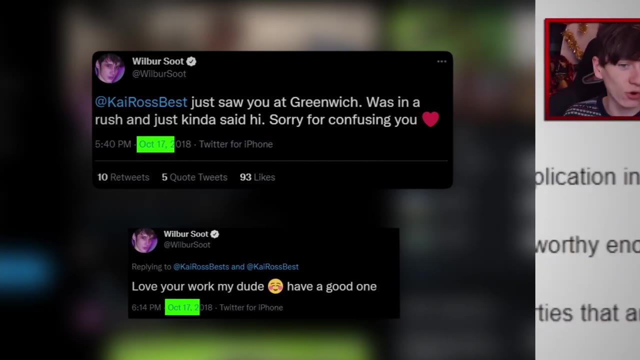 we see him tweet at Kai saying, quote: Just saw you in Greenwich, Was in a rush and just kinda said hi, Sorry for confusing you With a follow-up tweet about how he loves Kai's work- A very different tone from the email that we see. that starts this whole thing off. 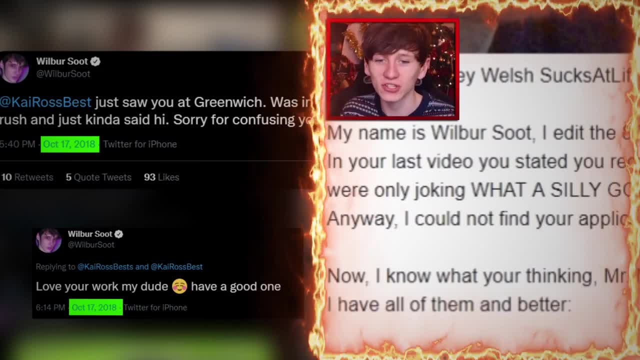 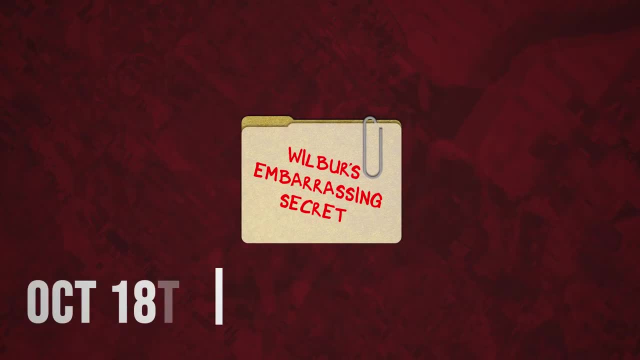 In short, what many people perceive as the beginning of this ARG, that first Jack video is really a few months into the whole thing. It also means that, whatever this quote-unquote embarrassing event was, it took place between October 18th and December 16th. 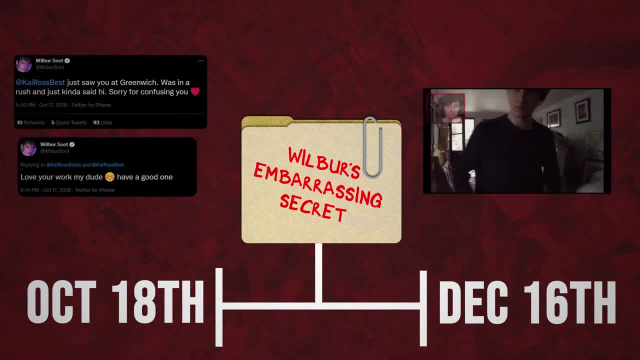 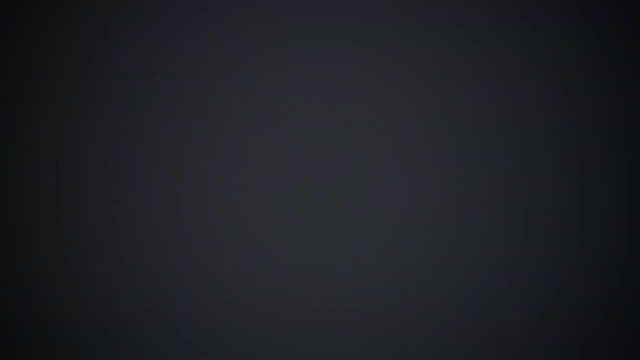 between the tweet complimenting Kai and the upload date of the video rant seen on Jack's channel. So certainly not the whole picture, but pieces are certainly starting to fall in place. The next chunk of clues actually came from Discord, where it seemed like Wilbur was using aliases to push things forward. 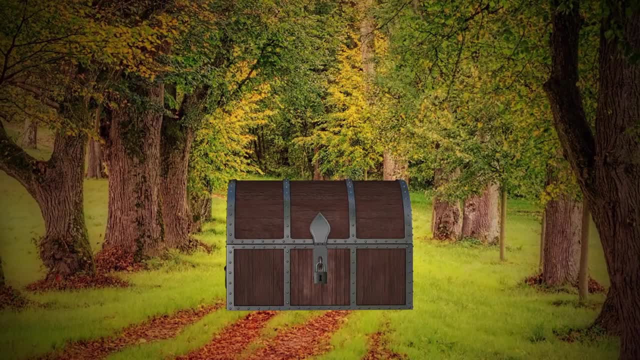 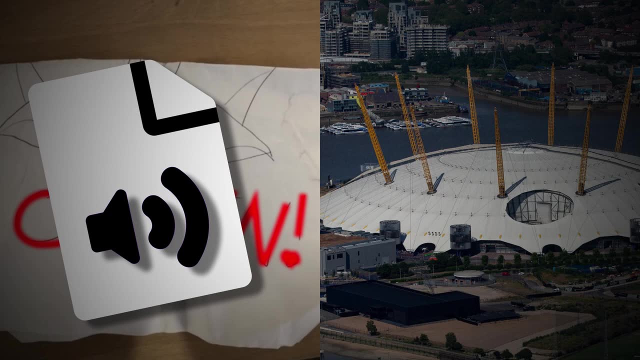 Via these presumed secret accounts, we learned about a hidden cache, IRL, which contained a drawing of London's O2 Arena And the word oxygen written beneath it. There were also audio files, stenographic decoders. broken links Like this one was really making people work. 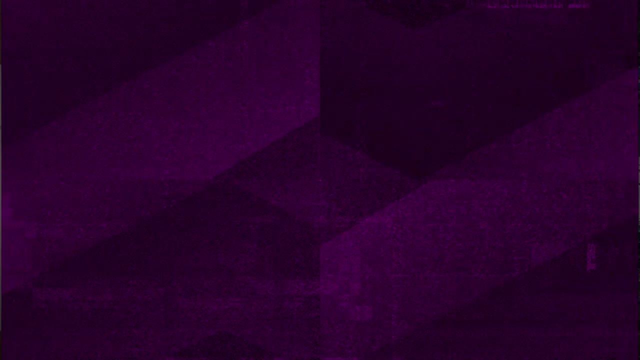 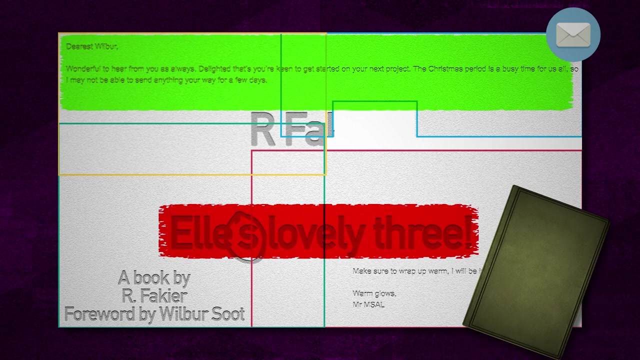 But through it all, you wound up with two major clues. First, this image, Which seems to be an email sent by Jack to Wilbur, mixed in with a book. title: Book cover: Elle's Lovely Three by R Fakhir. 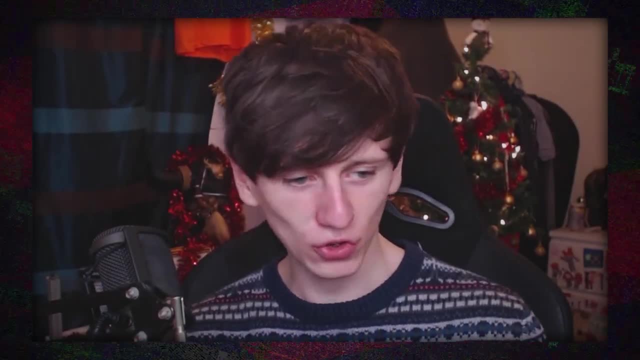 The second was yet another YouTube video where Jack syncs up and stares at a camera for about a minute or so. It's pretty boring stuff, but you know there has to be more to this right. Put the audio through a speaker. 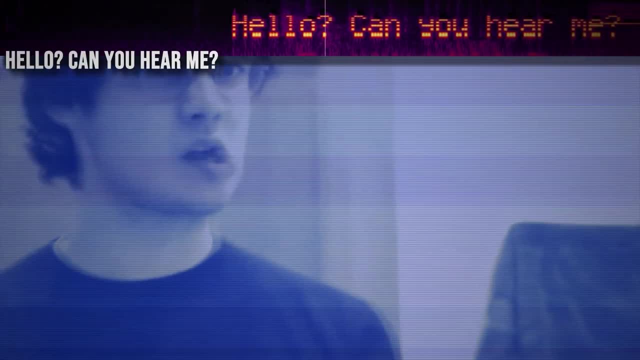 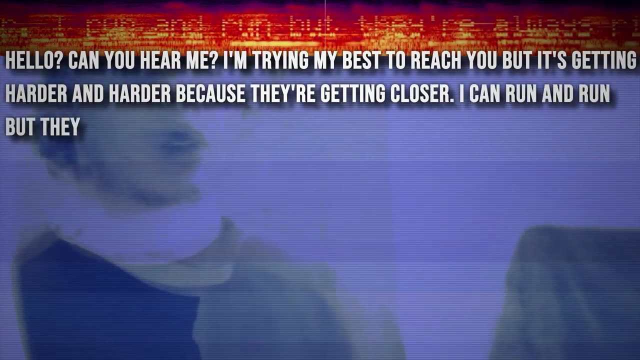 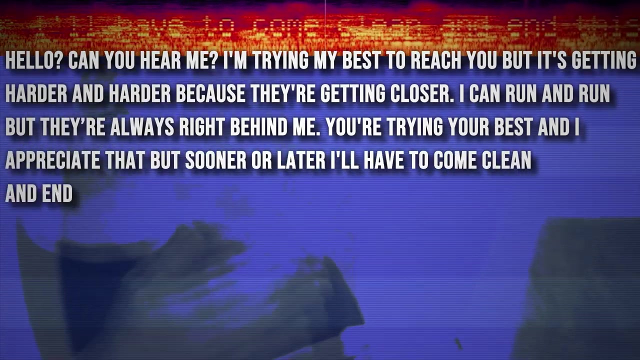 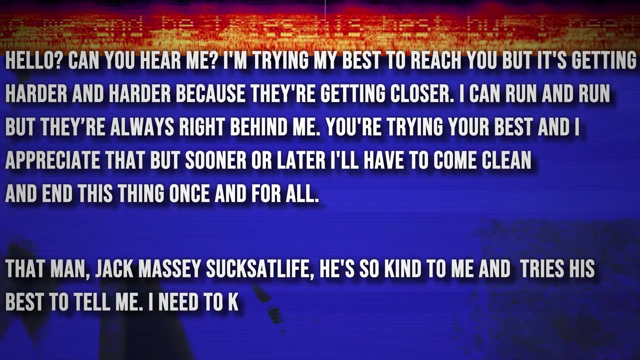 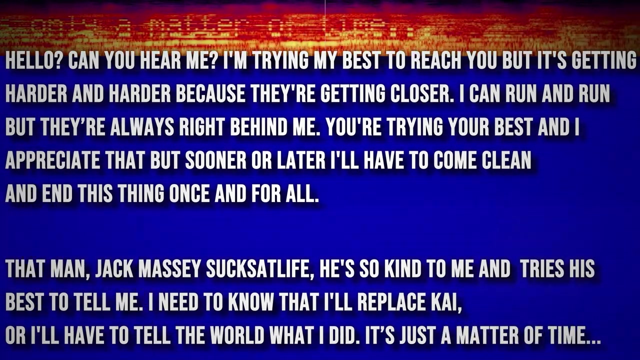 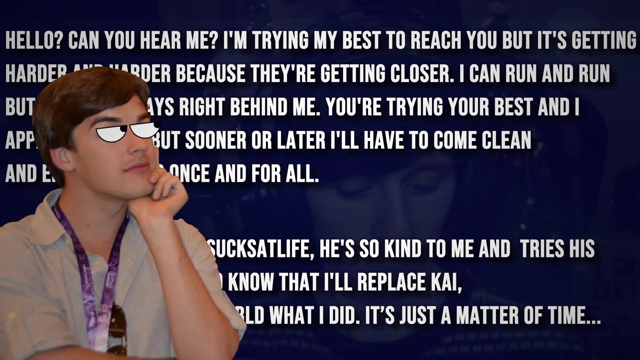 spectrogram and in the middle of the video you find some text. It's just a matter of time. It's emphasizing the parts of the story that we already know, but not revealing anything new. This becomes a trend that we'll see throughout the third video as well. 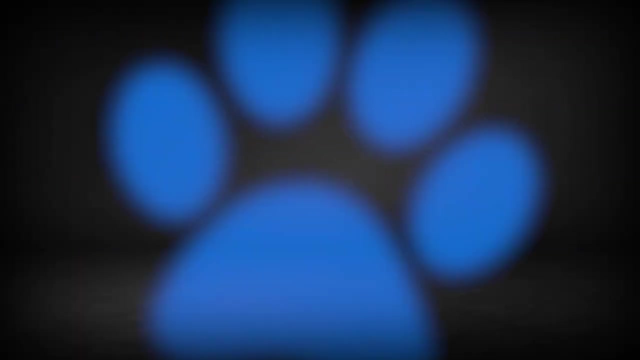 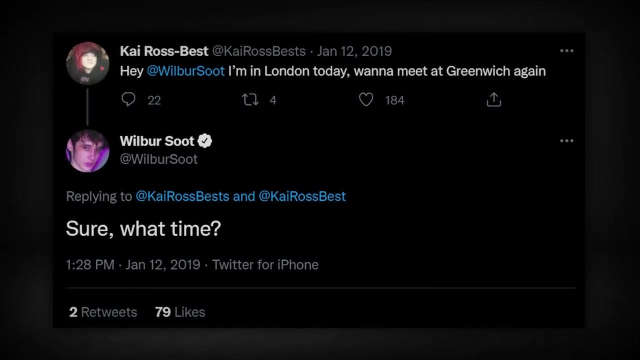 No, when it comes to big clues, at this point those actually shift over to Twitter. Kai and Wilbur seem to organize a meeting on the same day. the third video goes live. What exactly happens here between the two of them is unknown, but afterwards Kai's find a friend. location was ominously located in the middle of a river. 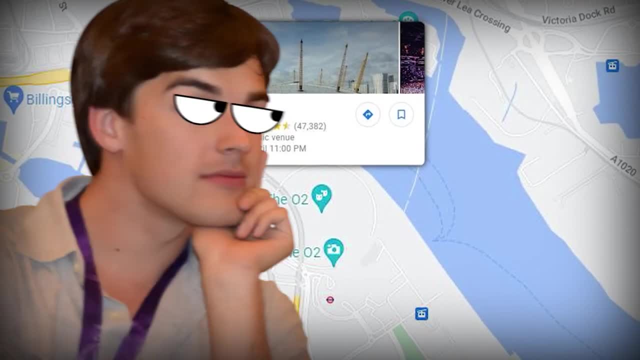 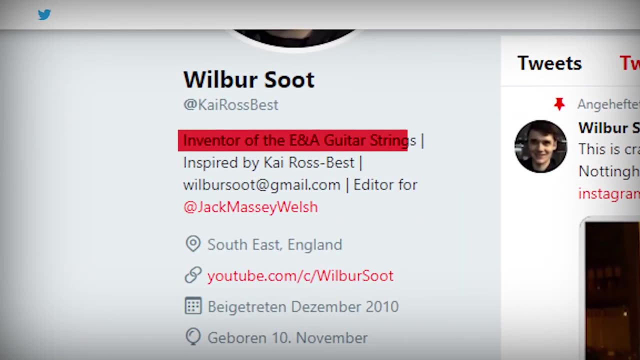 just downstream of the London O2 Arena. Suspicious, We're back there. Kai's Twitter account is also seemingly overtaken by Wilbur, His bio reading inventor of the ENA guitar strings. wilbursood at gmail dot com. 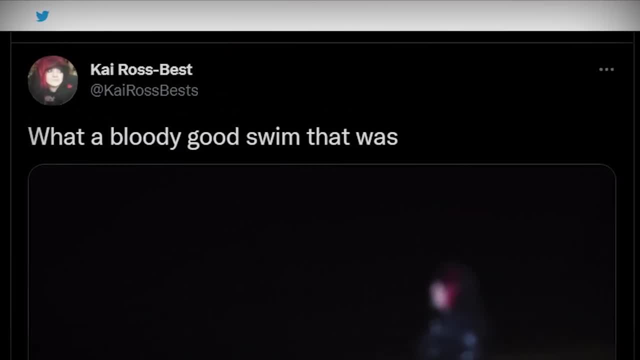 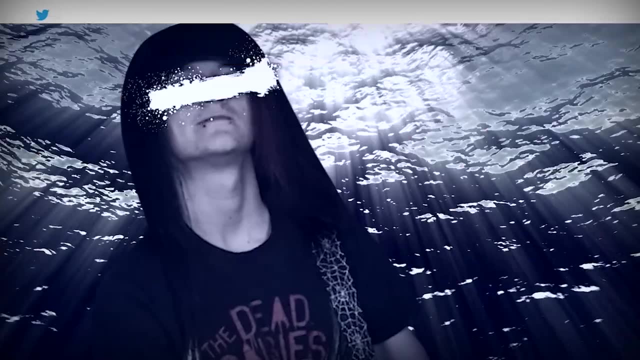 Two days later, Kai's Twitter returns to normal tweeting. what a bloody good swim that was, and that the water wasn't as bad as you'd think, but was bloody cold, though, to say the least. It seems that Wilbur attempted to get rid of Kai by getting him to swim in the river. 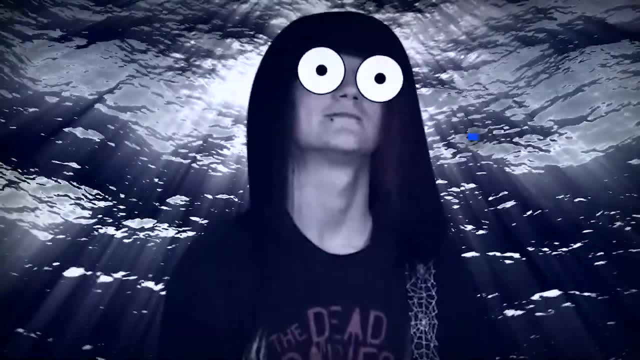 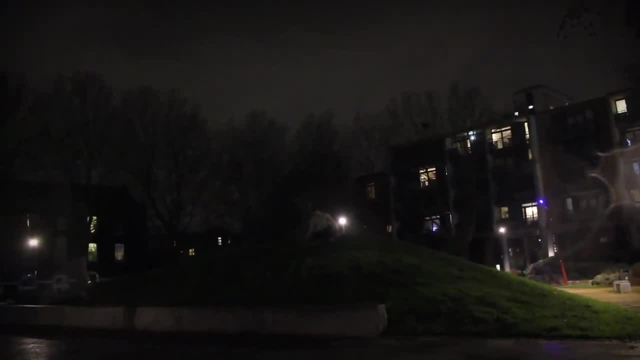 by throwing him in the river, something but Kai survived. Also, notice the detail about the water being cold, A direct callback to Wilbur Wilbur's repeated phrase that happens throughout this entire ARG. is Wilbur cold because he too was forced to swim in the water at some point? 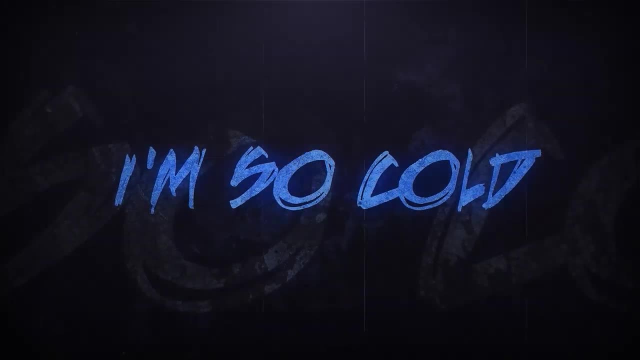 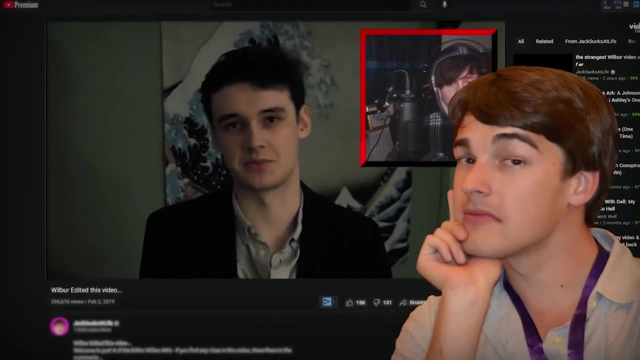 Maybe The I'm so cold phrase is so important that it becomes the major theme of the next set of puzzles in the series, starting at video four. Wilbur edited this video. Not much to talk about here. This step actually required a good bit of brute force to solve. 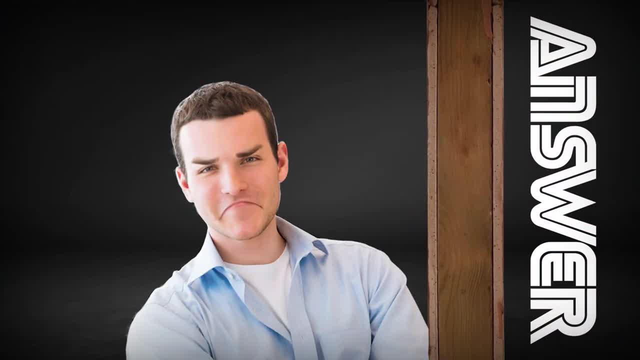 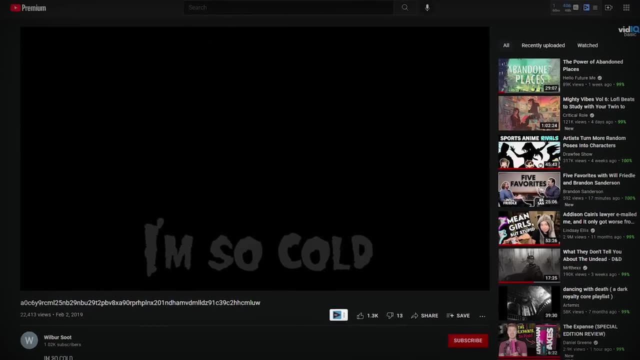 Brute force answering is when you basically just keep trying over and over again without any real hint as to the answer. Anyway, you eventually wind up at a video of Wilbur saying his classic catchphrase: Wilbur, I'm so cold, I'm so cold. 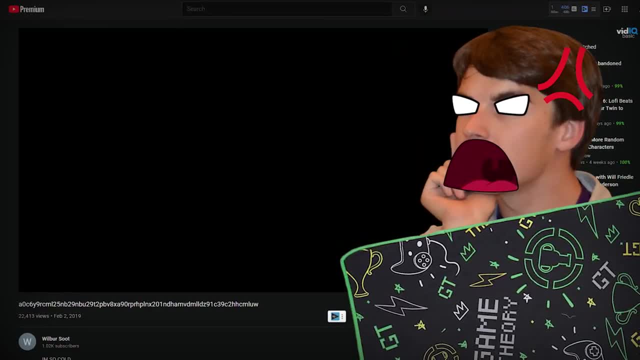 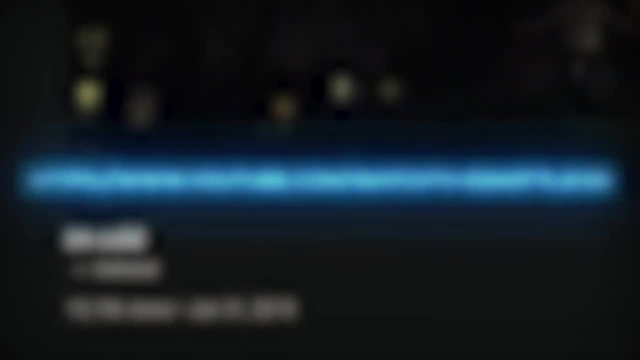 Over and over again. Seriously, can someone get this guy a blanket In the description of the video? we're given another base 64 code which translates to a backwards YouTube URL for another video titled. you guessed it. I'm cold. 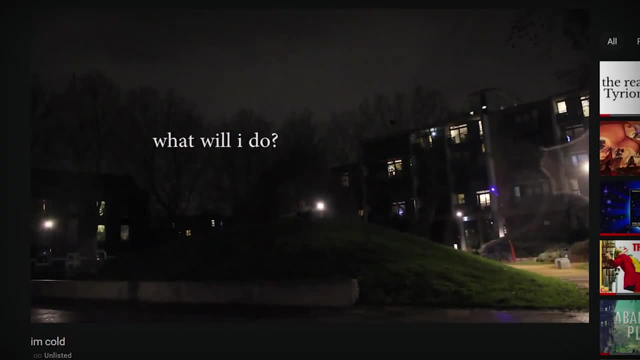 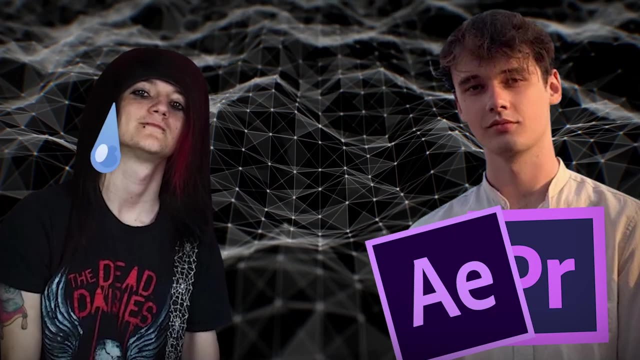 In this video we see text saying it's not forever, is it? What will I do? And, of course, I'm so cold. These are all comments on the fact that in the overarching story, Wilbur has just gotten the editing job over Kai. 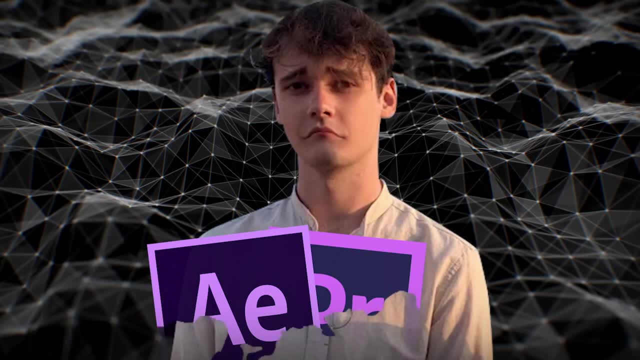 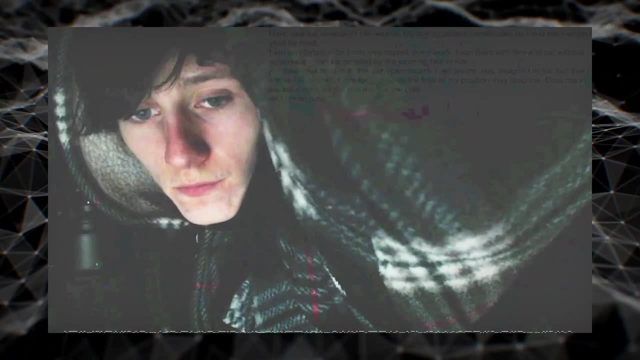 But clearly he knew that even though he had won temporarily, it wouldn't last. But clearly he knew that even though he had won temporarily, it wouldn't last. A poem found in an imager photo around this time also backs this up. I can paint with film and cut without scissors. 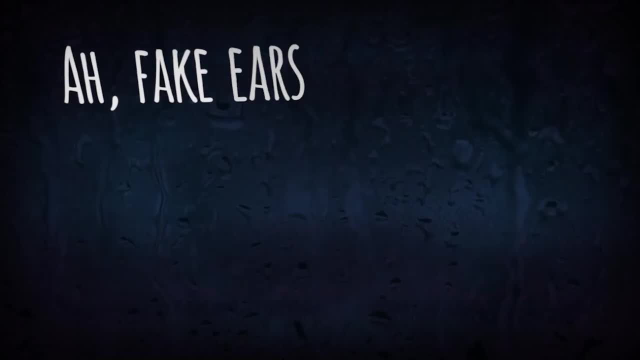 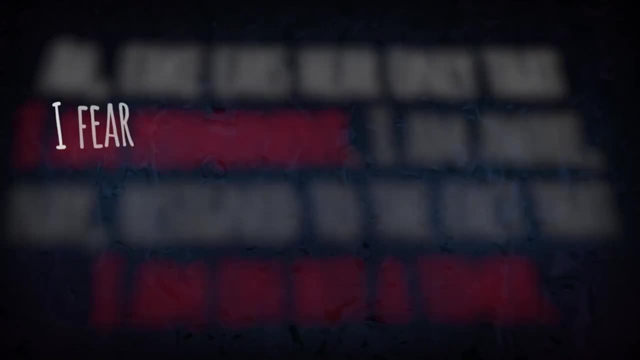 and not be hassled by the looming fate of Kai Ah. fake ears hear only that I am permanent. I am aware, nay, resigned to the fact that I am on but a timer, I fear myself as the loss of my position may drop me. 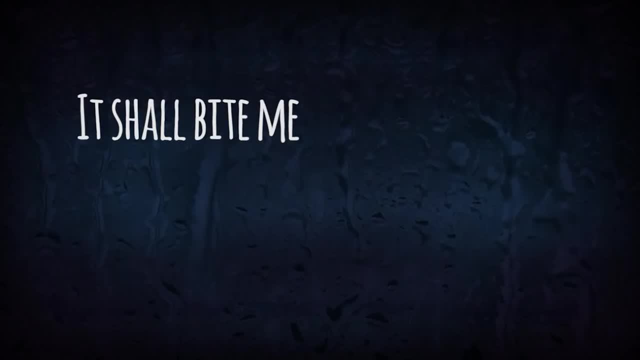 drop me in the wasteful void. It shall bite me like the cold And I'm so cold. Between the Edgar Allan Poe references and all this fancy Shakespeare. Between the Edgar Allan Poe references and all this fancy Shakespeare. Between the Edgar Allan Poe references and all this fancy Shakespeare. 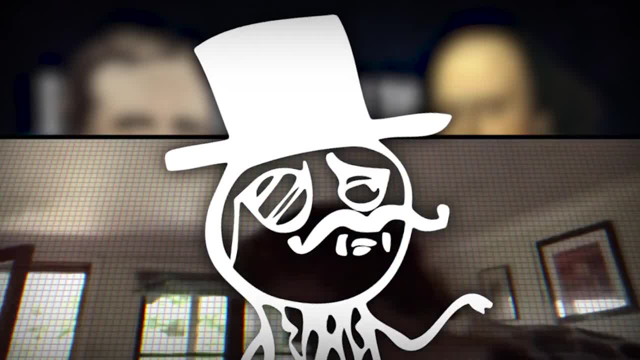 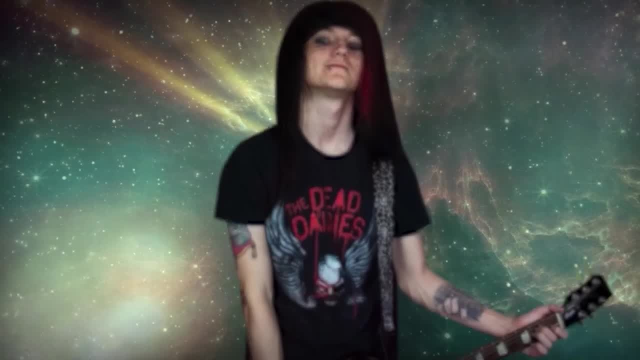 talk, you can tell that this one is a classy ARG. Anyway, all of this is him knowing that this isn't a permanent fix for the problems that he's caused. It's merely a distraction. Kai will return, and if Jack removes Wilbur from the equation, 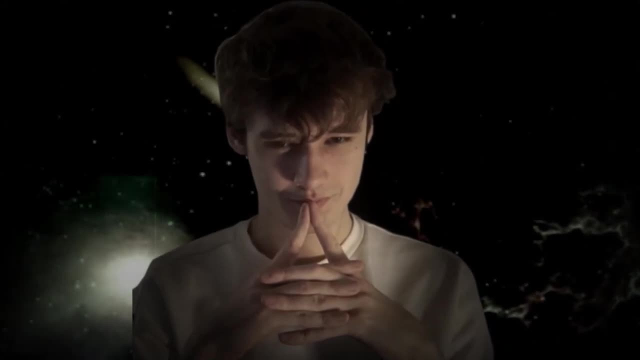 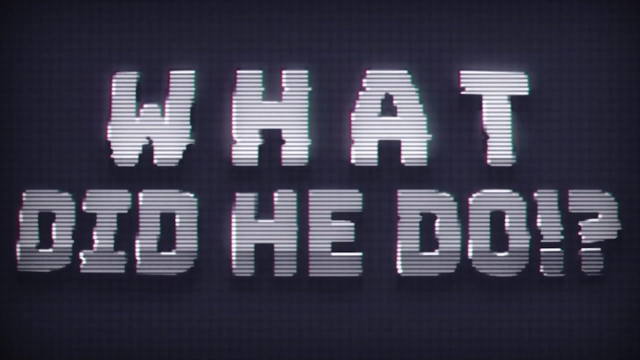 then he'll be left alone in the void, with nothing to distract him from what he's done. So what is it? What did he do? And this, you see, is why the ARG is currently unsolved. No one has that core answer. 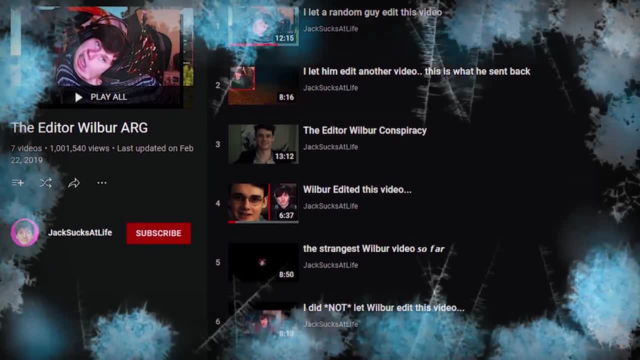 There are more videos after this. more references to being cold, more drama, as There are more videos after this. more references to being cold, more drama, as There are more videos after this. more references to being cold, more drama as. loses the job back to Kai and plenty more codes to solve. 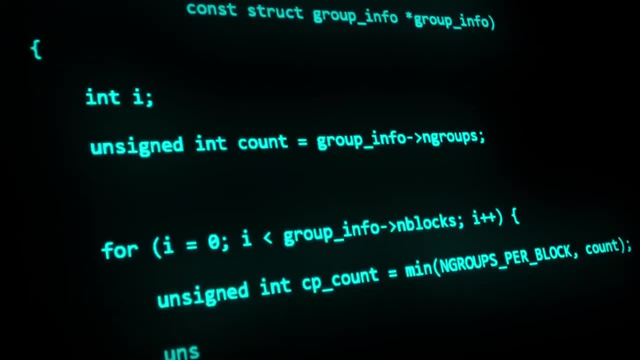 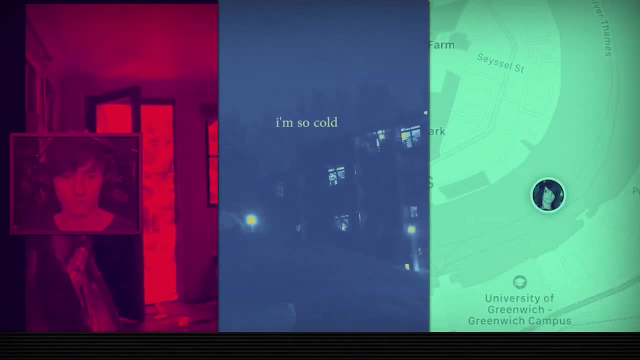 but to me and anyone who knows this mystery, the question everyone wants closure on is why? Why is Wilbur on the run? Why is he so cold? Why does he want Kai silenced? What is the big secret? At first, I started to pick at the loose threads of clues that no one knew what to do with. 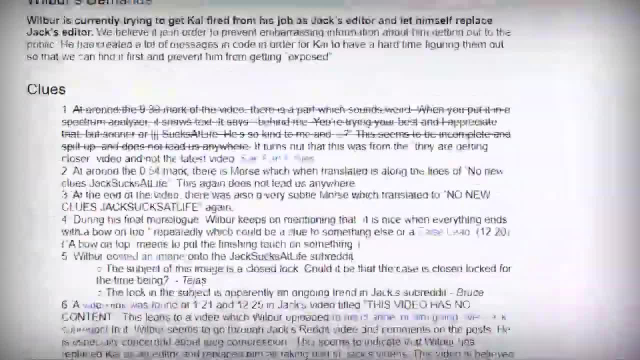 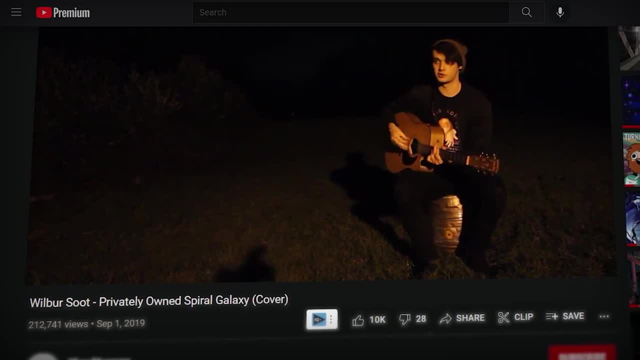 or at least that didn't have clear endpoints on the massive Google Doc that the fan community made. There was, of course, the Wilbur Soot music video, privately owned Spiral Galaxy, which just kinda appeared at one point in the middle of the ARG. 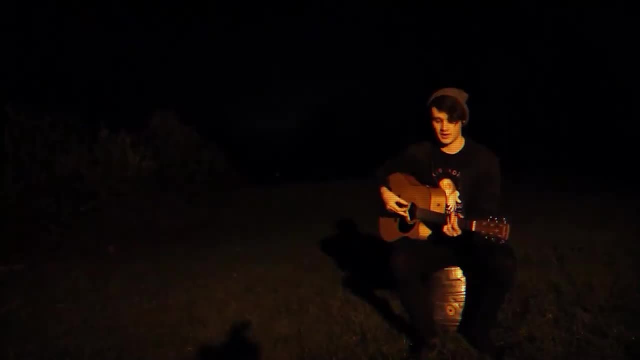 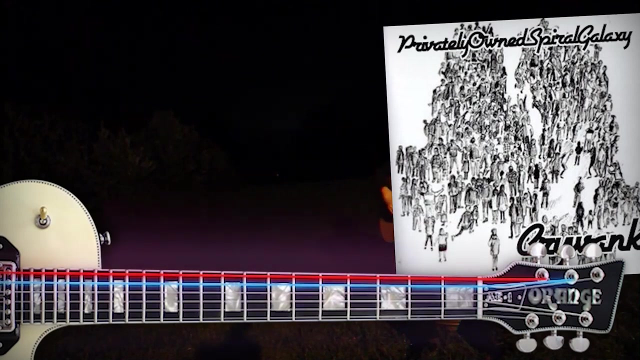 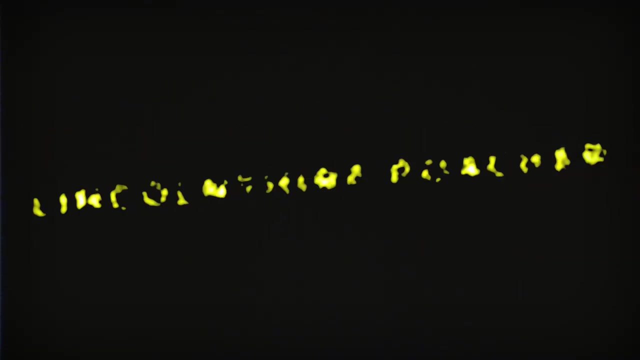 In this video, Wilbur sits on a keg in a field and plays a slightly modified cover of the song, privately owned Spiral Galaxy, notably playing the song almost entirely on the E and A strings, the ones that he claims to have invented. If that wasn't suspicious enough, at 2.27, the video cuts away suddenly to play the Lincolnshire Poacher tune. 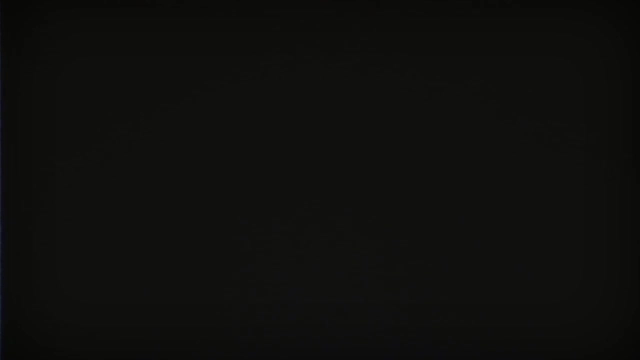 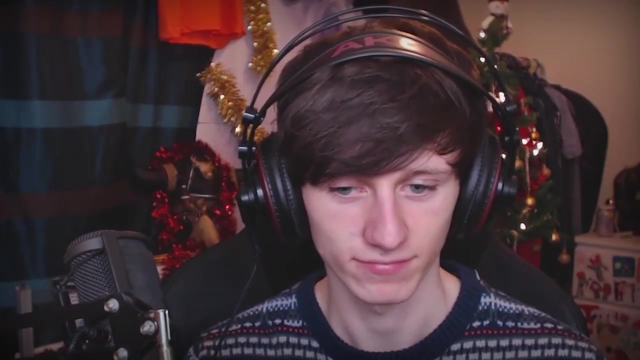 So clearly this video has something important to hide. in the greater ARG and after being involved in the Petscop ARG for so long, one of my first instincts was synchronization. Remember that video I mentioned earlier, The suspicious one Where Jack stares at a camera for a minute or two and nothing really happens. 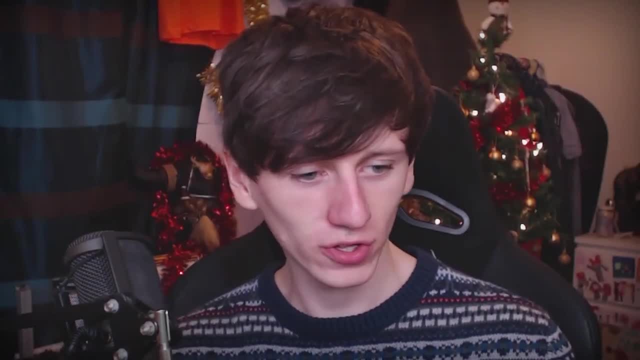 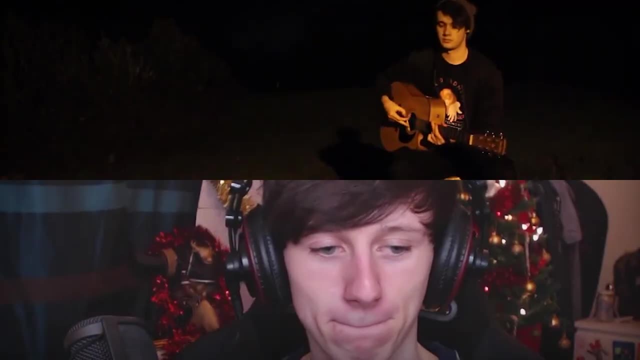 Well, it starts with Jack saying: Okay, I'm syncing up One, two, three. One two, three Seems like the perfect opportunity to sync some videos up, So I tried it and, wouldn't you know, they sync. 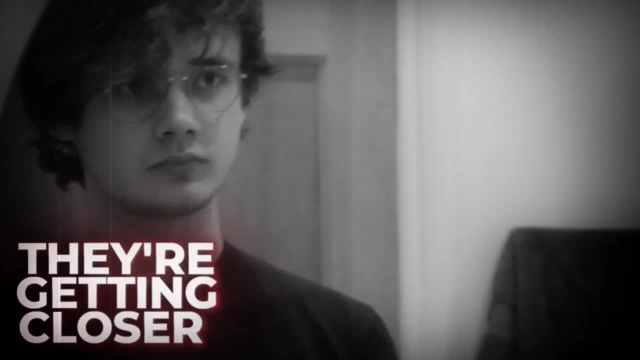 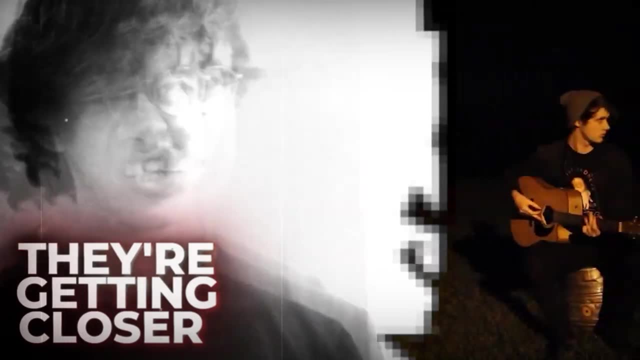 At 2.21, in There, Getting Closer Jack, is suddenly replaced by a black and white video of Wilbur staring into a bathroom mirror, while digital sounds play in the background. At 2.27, exactly the song gets to the same point. the digital tune plays in privately owned Spiral Galaxy. 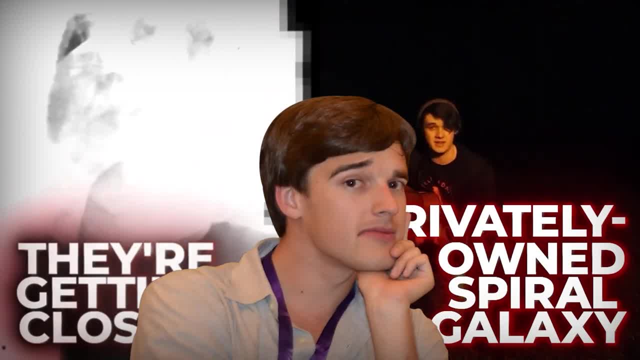 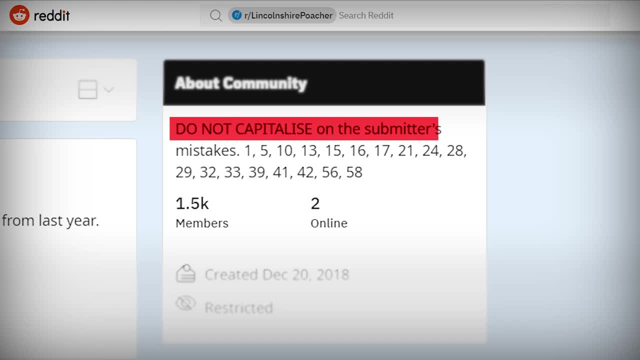 It's cool, but what? It was? a new finding that ultimately led to nothing. as far as I could tell, In the rlinkenshirepoacher subreddit there's a cryptic hint in the information bar. do not capitalize on this poster's mistakes. 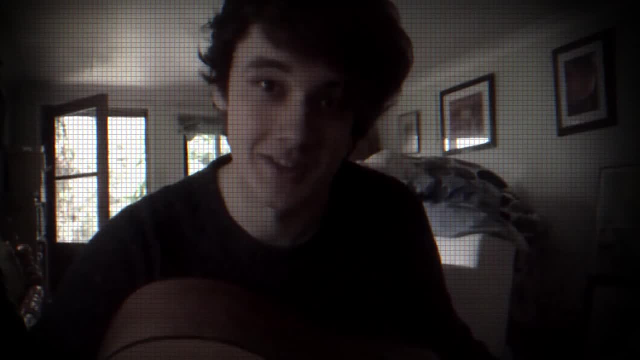 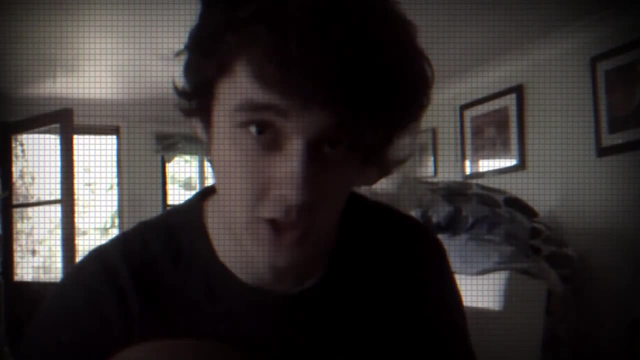 and in the first video of the ARG, Wilbur claims to be suffering from frostbite and apologizes for not being good at guitar. as a result, My fingers are suffering from hypothermia at the moment, so if I'm not very good, my apologies. 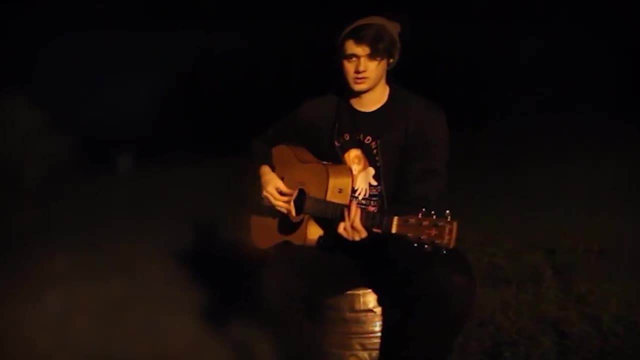 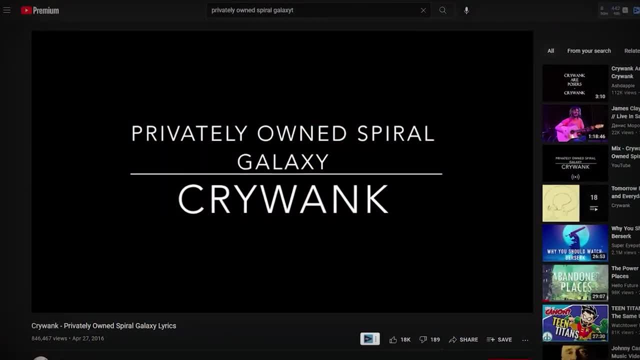 And those are telling me what to quote- unquote- not capitalize on. And those are telling me what to quote- unquote- not capitalize on. Well, after listening to the original version and comparing it with Wilbur's version, I found three different notes that just seemed out of place. 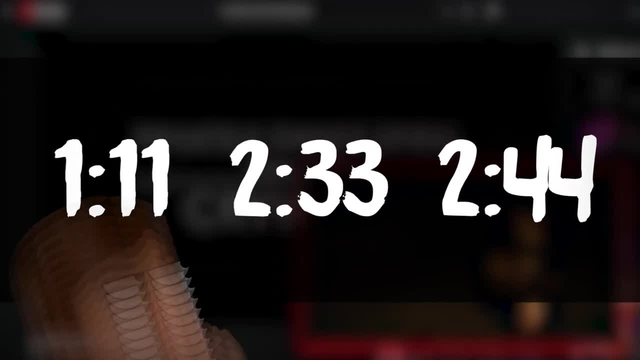 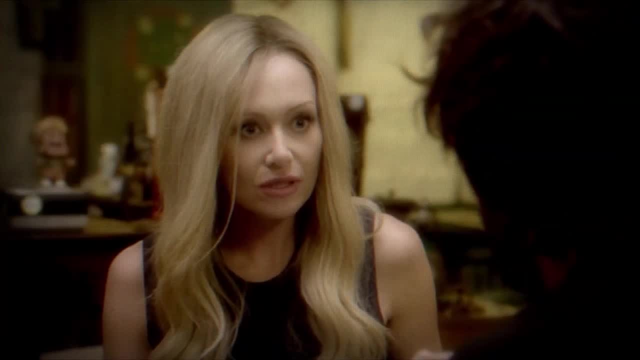 One at 1.11,, one at 2.33, and one at 2.44.. Are these repetitive timestamps just the product of me looking too deeply into one puzzle, or do they actually mean something? That's not a coincidence. 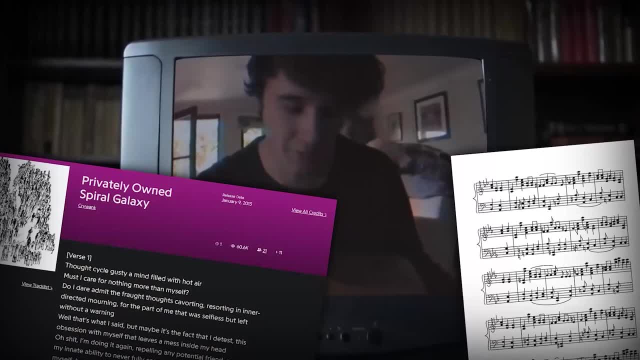 I don't know. I tried a bunch of things: the lyrics, the letters, whatever. I still seem to be missing a step, a clue, something. And I still seem to be missing a step, a clue, something. And I still seem to be missing a step, a clue, something. 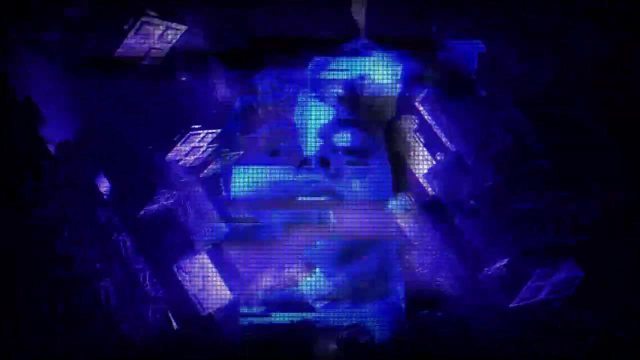 And I still seem to be missing a step, a clue, something. I could just sit here and list off more of the random rabbit holes that I looked down, but the end result was always the same, While I certainly had some new findings here and there. 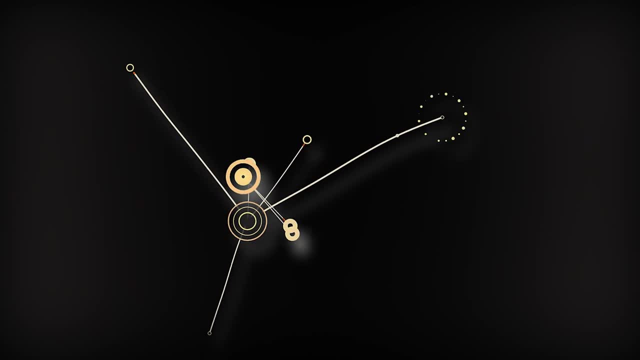 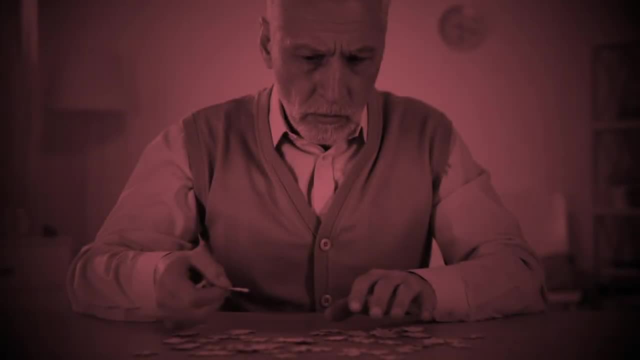 none of it was earth-shattering. Nothing was truly connecting the dots in the way that I would imagine those dots connecting. Wilbur was ultimately right with his phone call to me. I couldn't solve it all, But here's the thing: Just because you don't completely solve every puzzle doesn't mean that you can't win the game. 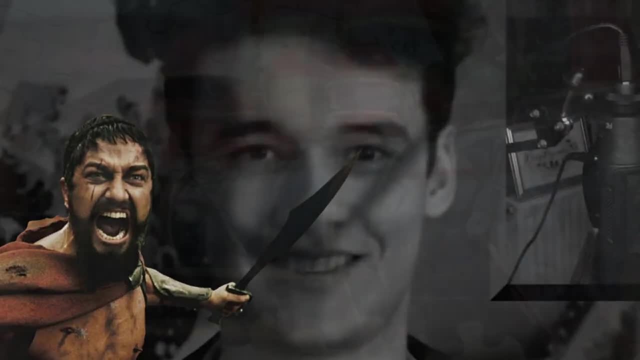 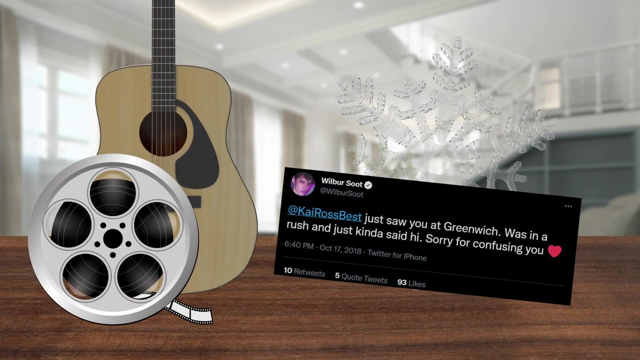 Wilbur may have won some battles here and there, but he hasn't won the war. Just like you can know the image hidden on a puzzle without having all the pieces, I think there's enough clues on the table at this point to actually solve the main mysteries. 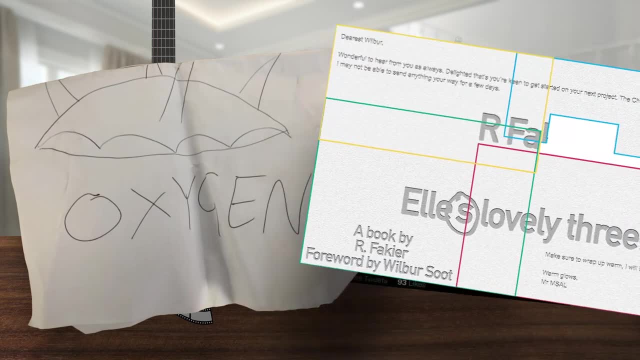 of this thing. I think I know what happened at the O2 arena. I think I know who the Fakiers are- There's actually two of them. we'll get to that- And I think I know why everyone is so darn cold all the time. 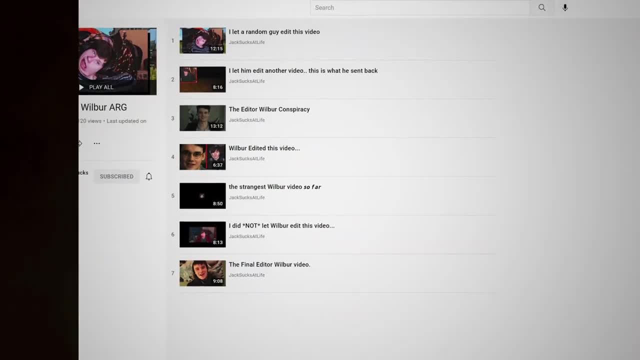 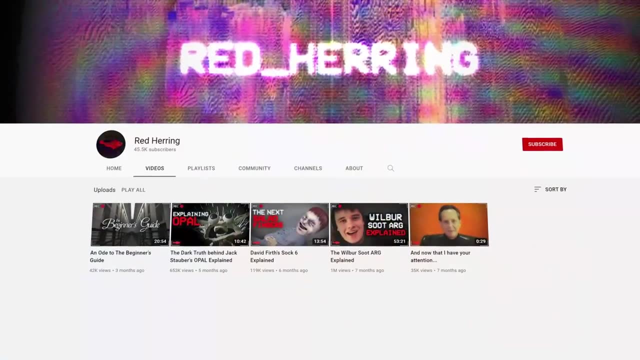 So, finally, it's time to talk theories. As you can probably imagine, in absence of a definitive conclusion to the ARG, Wilbur's communities developed some guesses to fill in the blanks of the story. The first comes from the YouTube channel, Red Herring. 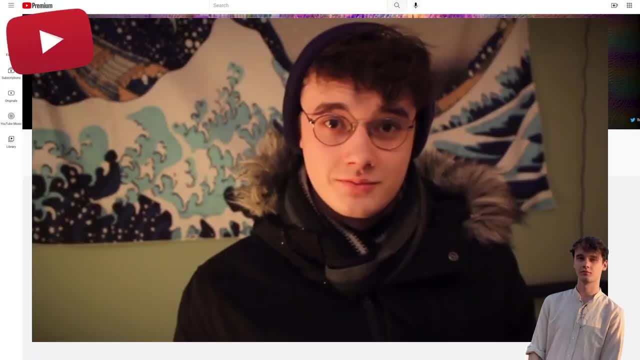 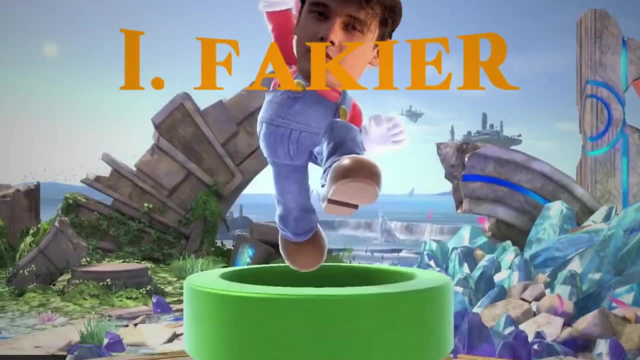 They propose that R and I Fakier are actually two different personalities of Wilbur And yeah, I kind of skimmed over it. but at one point in the ARG a new challenger enters the fray. I Fakier On Reddit. Wilbur suddenly makes a random comment on a post, just saying: 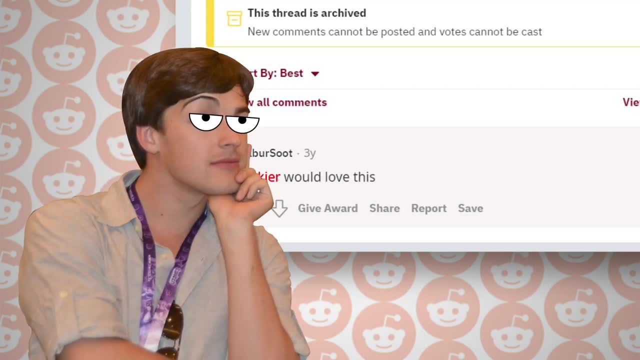 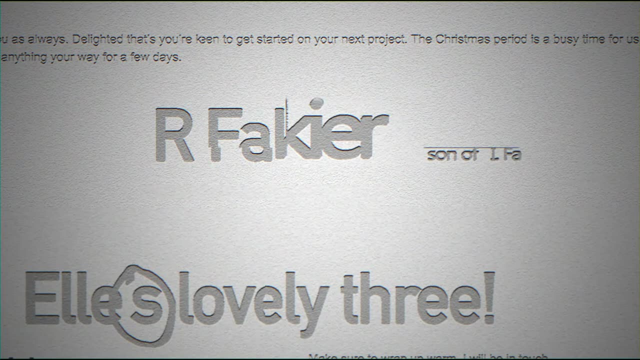 I Fakier would love this. I Fakier, I thought it was just R. you know the guy that wrote the book from earlier. Well, we learn later from R Fakier's completed book cover that R is the son of I Fakier. 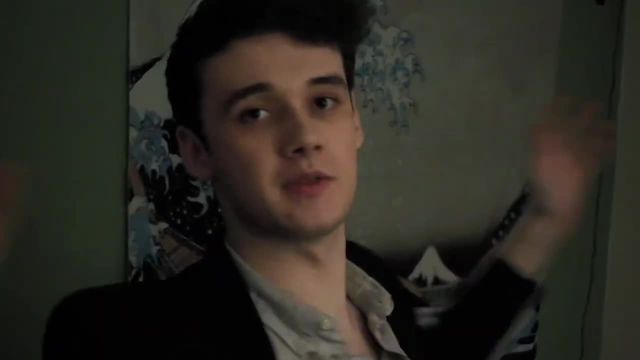 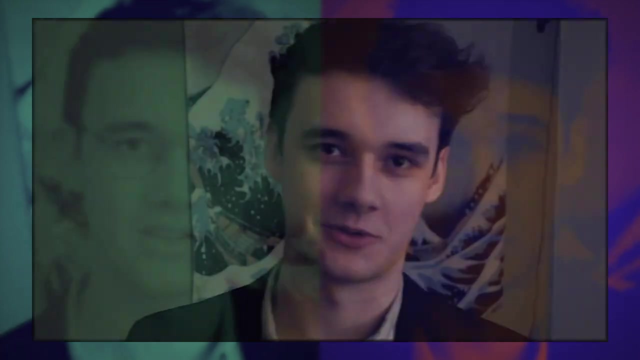 which is also an anagram for Fire Kai. Very clever, Anyway. throughout the entirety of the ARG, Wilbur is seen both with and without glasses, sometimes even switching Between wearing and not wearing them in the same video, And when he switches, his demeanor seems to change as well. 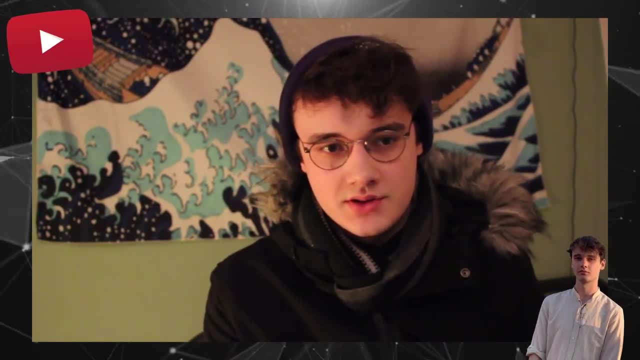 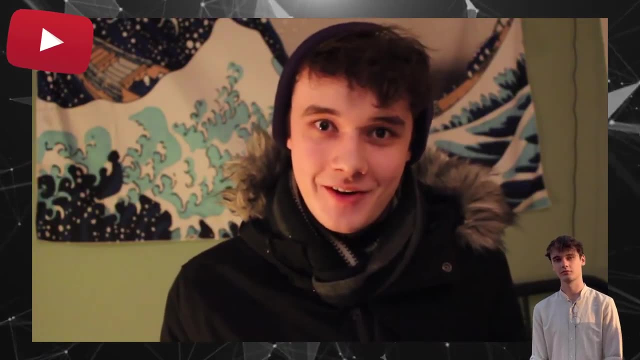 When they're on he comes across as obsessive, but calmer and put together. It's nice when things end with a bow on the top. When they're off, he becomes erratic, impulsive and aggressive. We love our deadlines here. 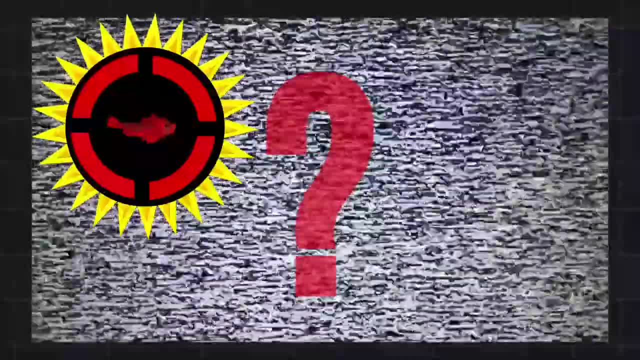 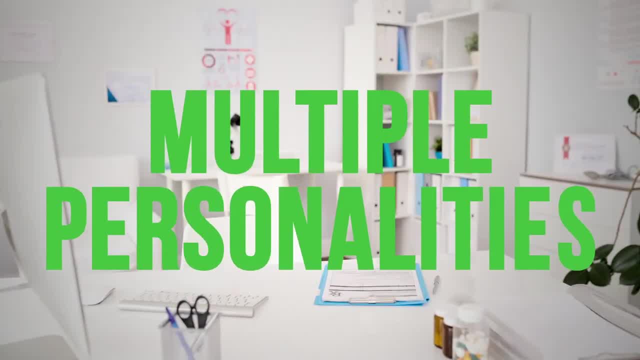 We love our deadlines. We love them. The theory goes that whatever traumatic event is at the core of this ARG, it may have caused Wilbur to develop dissociative identity disorder, more commonly known as multiple personalities. This condition is commonly the result of trauma. 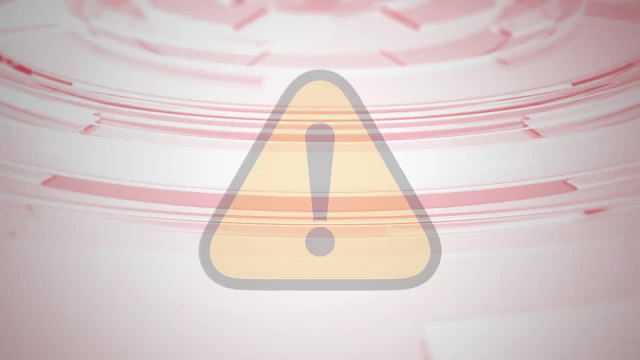 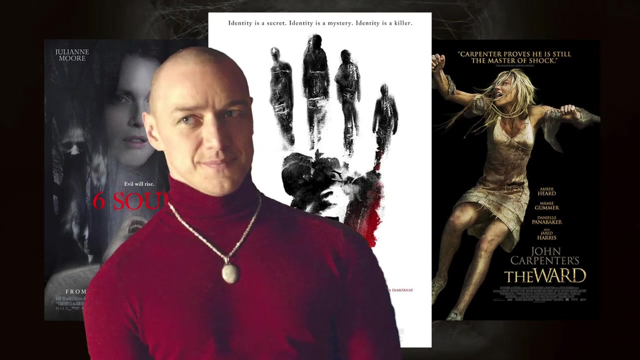 as the brain actively tries to avoid bad memories. And let me just put in a disclaimer here: This is a real condition that is often very negatively and poorly portrayed in media outlets, usually with scary people who are serial killers being the ones that suffer from it. 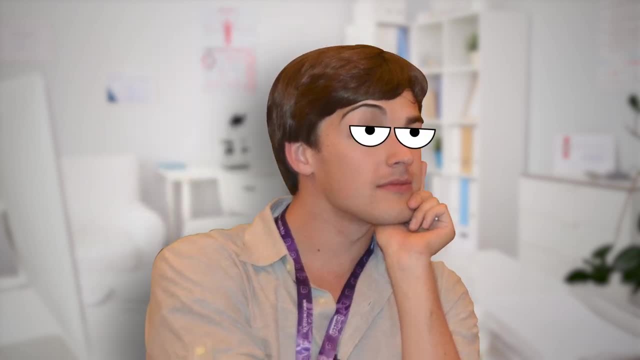 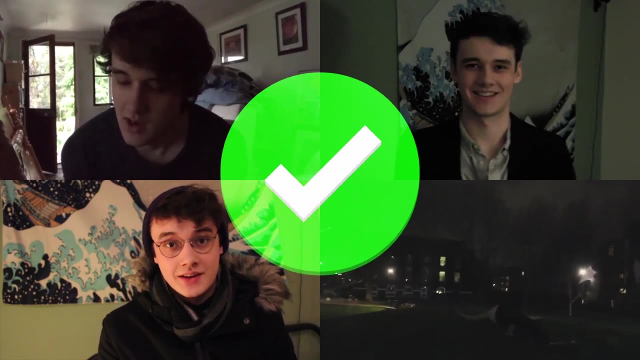 So please do not fall victim to that stigma. It is not true, It is just made up and over sensationalized. Anyway, applying this idea to Wilbur's behavior throughout the series, a lot of things seem to fit. Wilbur only ever talks about the embarrassing incident when he isn't wearing glasses. 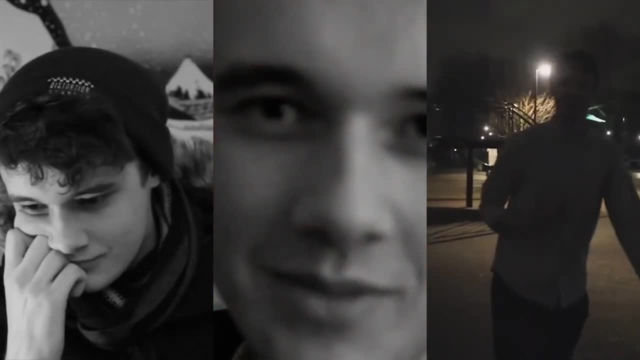 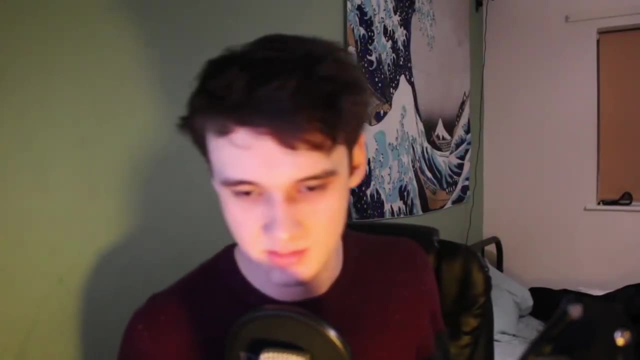 Same thing when he's demanding the firing of Kai or celebrating getting the job as editor: All No Glasses. During a Reddit review video, Wilbur looks for his reading glasses and then states: I've never owned reading glasses, Implying that this persona isn't aware of the other. 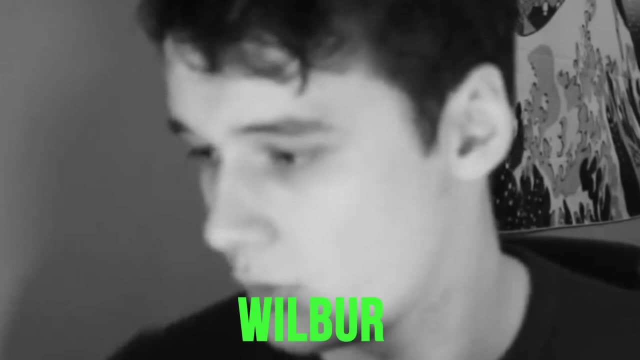 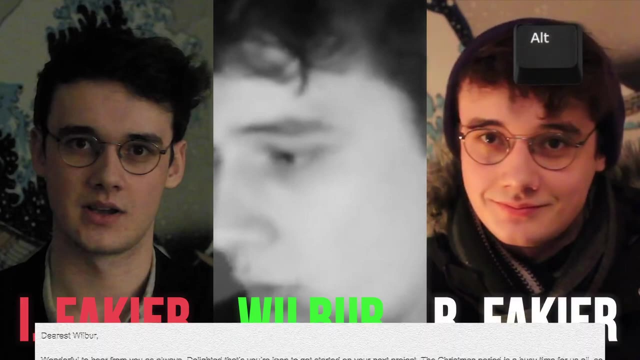 This is the real Wilbur, the one who wants to escape, who wants to forget. This is iFakir. Our Fakir, then, is the alt personality, the other persona, the son or product of iFakir. 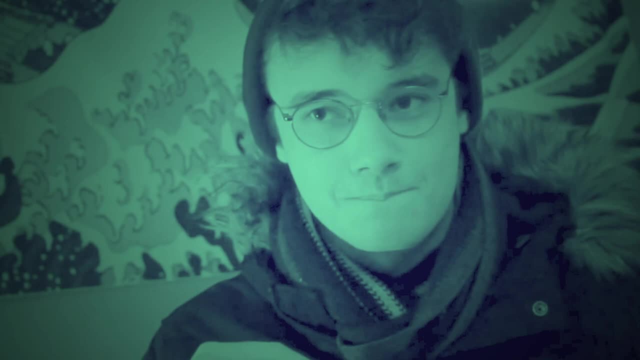 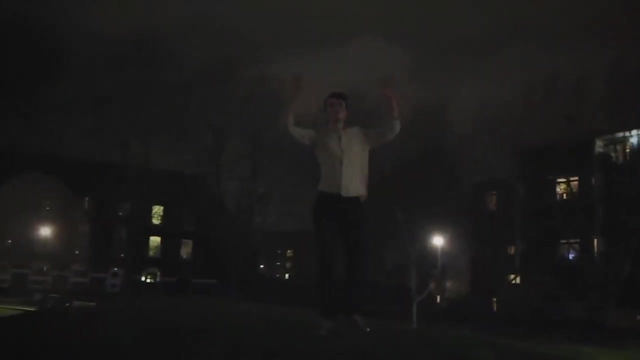 It's a persona that's like, more emotionally distant, more collected. Honestly, I think that this is right. The evidence for it is too hard to deny and it explains a lot of the weird Fakir stuff, but clearly it's not the whole story, because we still do not know what is the inciting incident. 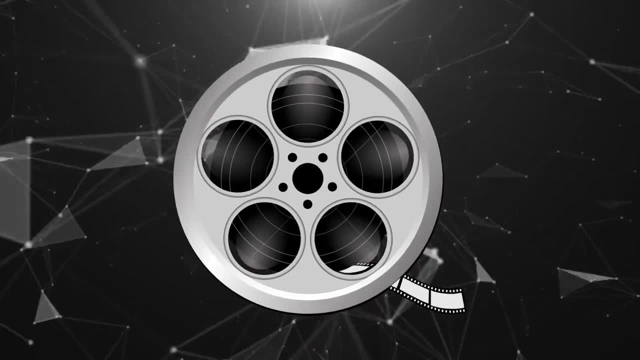 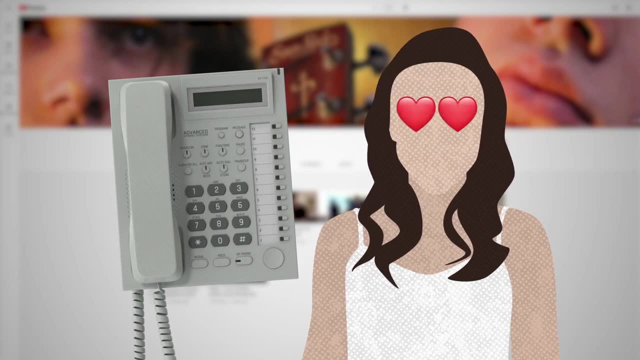 Well, for that we need to introduce one final video, one brought to light by online user Christian. This video on Wilbur's music channel features a voicemail from a girl who asks Wilbur out on a date. We haven't been on a date since like forever. 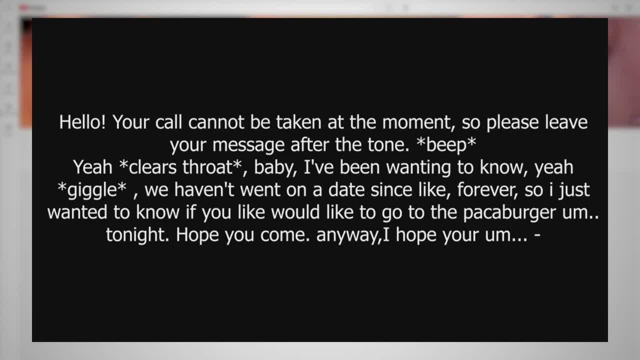 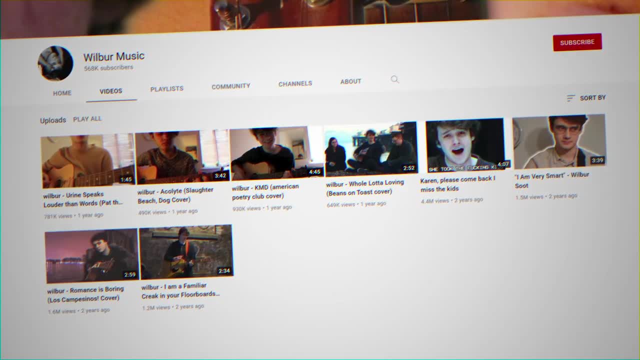 so I just wanted to know if you would like to. And that's it. We never hear about this girl again. It is a one-time, random event that, for followers of Wilbur's work, seemingly goes nowhere, and it's this random phone call. 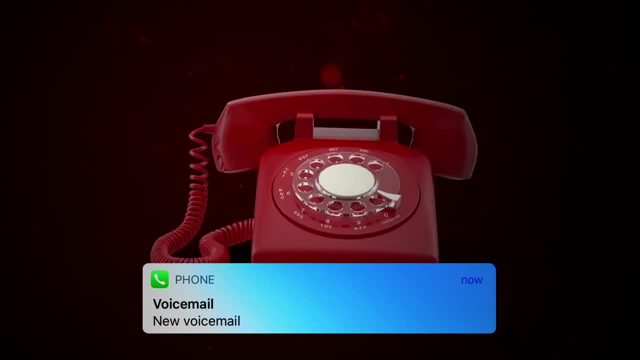 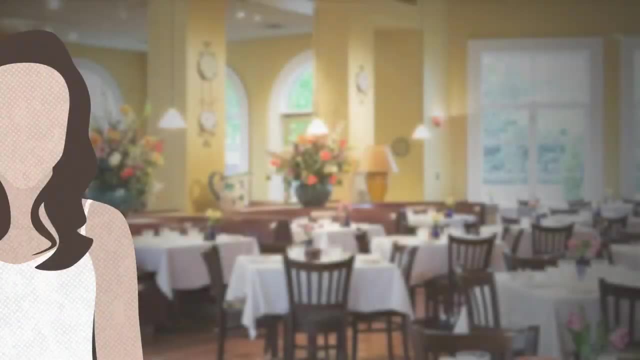 this out-of-nowhere voice message that I believe serves as both the beginning and end of the Wilbur ARG. Using both theories as a base, I think I've got the complete picture. This mystery girl asks Wilbur to meet her at a burger place. 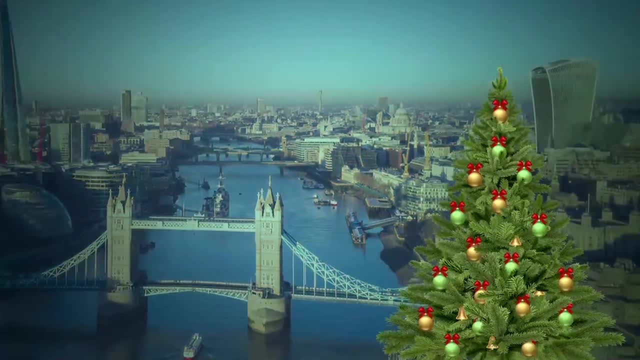 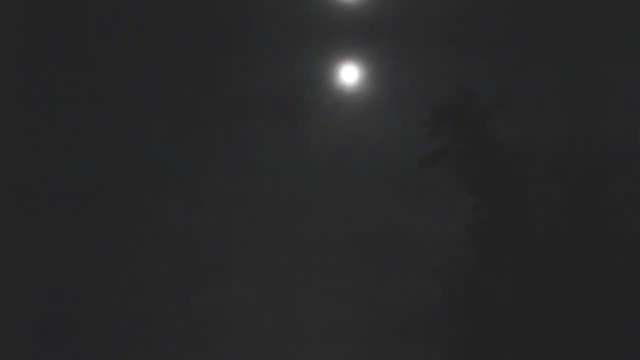 which let's assume is in Greenwich near the O2 Arena sometime in December. Remember this has to have happened before December 16th but after October due to his relationship with Kai changing. It also links to the poem The Raven that kicked this whole thing off. 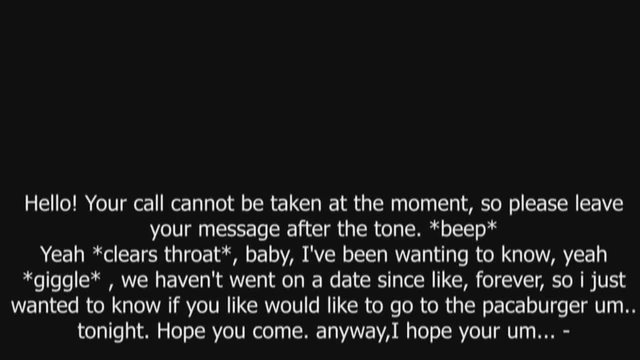 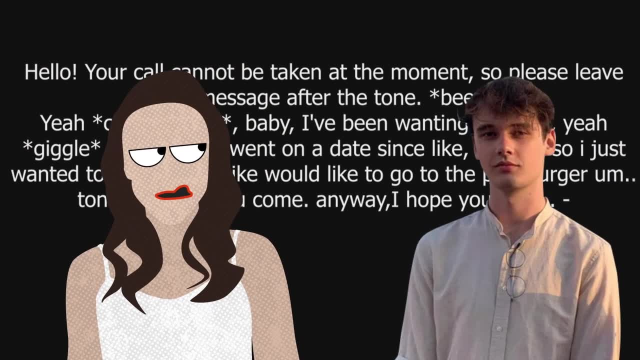 Distinctly. I remember it was upon the bleak December. The voicemail from this girl seems to be quite awkward, but to me it comes across almost as mocking Jeez. mocking is social awkwardness. It's kind of like when you're in school and the popular girl pretends to be interested in you. 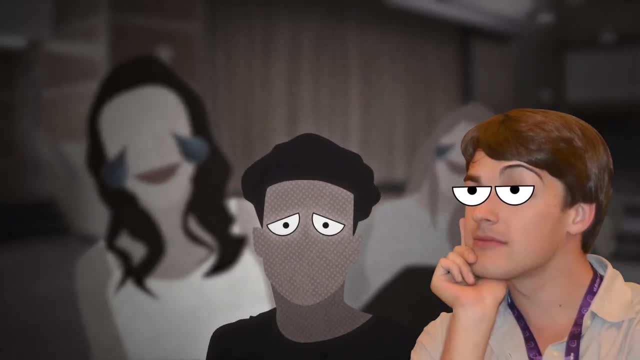 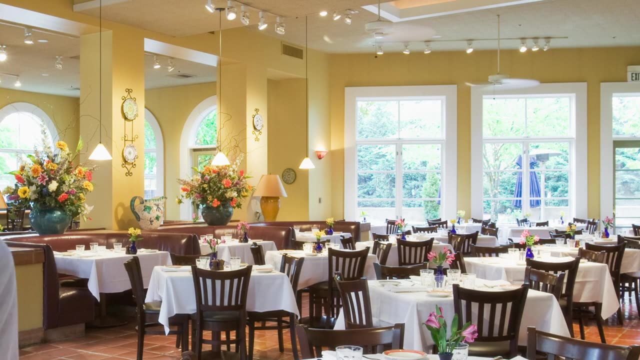 and then it all comes out as just being a prank. I have a sneaking suspicion that this might be what happened here. Wilbur's social awkwardness meant that he wasn't able to read the situation correctly. he clearly likes the girl, and so he showed up. 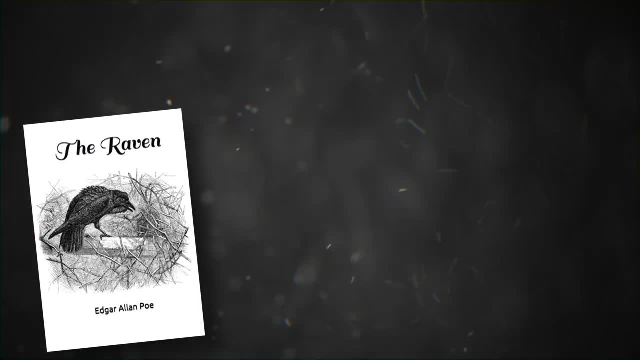 Which links in our first Edgar Allan Poe poem from the ARG Eula Lee, A poem about a lonely man finally feeling whole thanks to a woman Quote: I dwelt alone in a world of moan. Now doubt. now pain come never again. 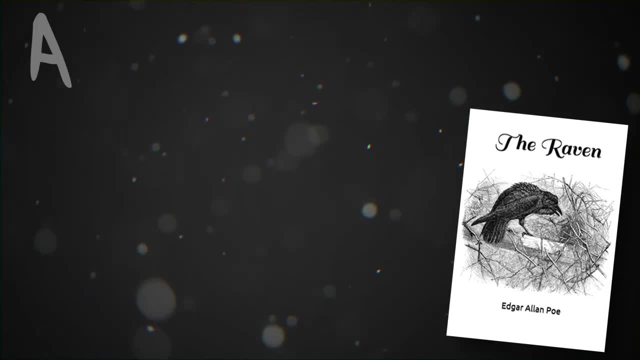 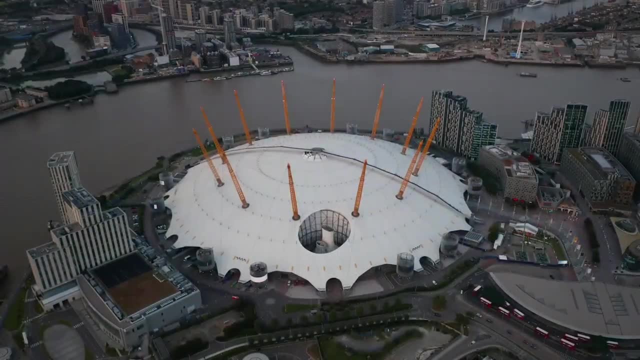 This then leads us to a second Edgar Allan Poe poem. Annabel Lee Quote again: I was a child and she was a child in this kingdom by the sea. By the sea, in this case, the Thames River, and referring to both himself and a mysterious girl. 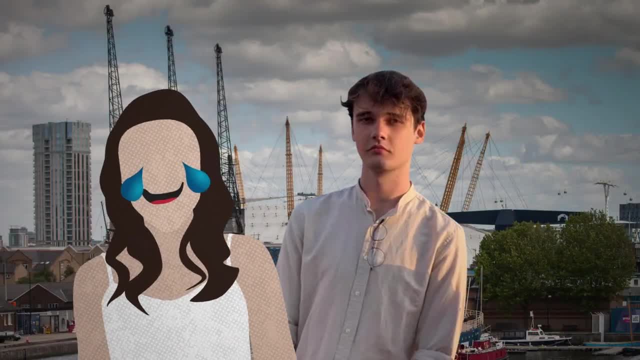 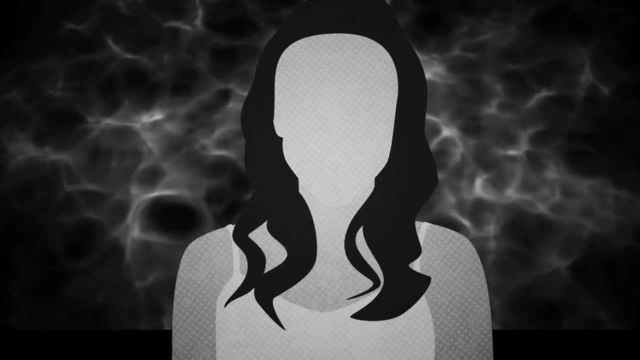 However, when he does go, she reveals that it was all a joke, causing this moment to be marked in Wilbur's mind as embarrassing. He was humiliated and, in a moment of rage, pushes the girl, which causes her to fall off the edge and into the cold water of the Thames below. 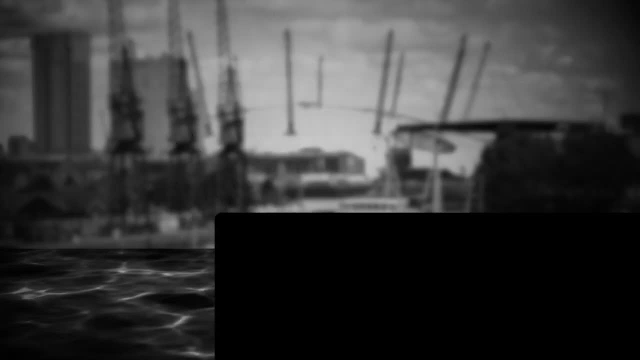 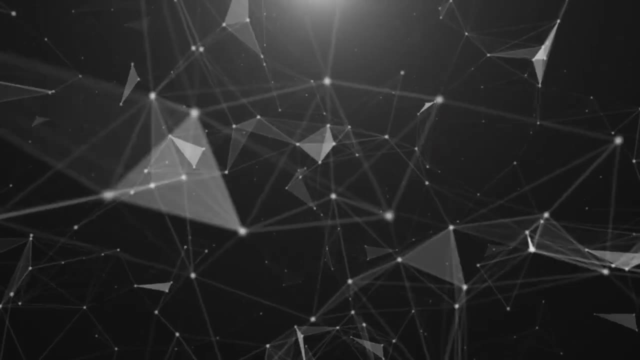 Wilbur panics. he dives in to try and get her out, but he's unable to. She's not able to swim and slowly begins to drown, with the last thing Wilbur hearing being the words: I'm so cold. This explains the pictures of the O2 arena and the word oxygen written in the geocache notes. 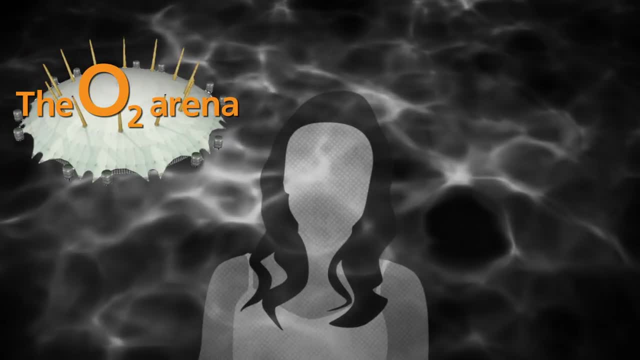 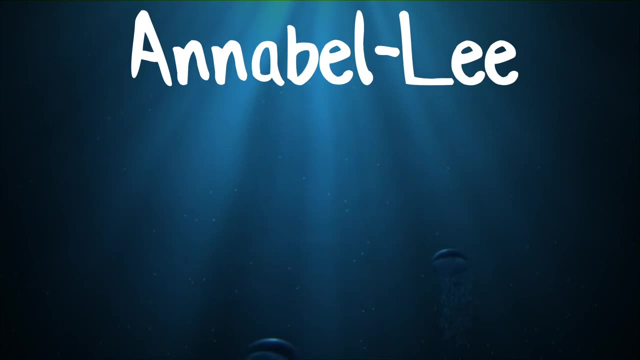 She drowned in the Thames near the O2 arena, lacking O2 or oxygen, Which also fittingly ties into that Annabelle Lee poem again, where the girl dies cold and wet Quote That the wind came out of the cloud by night. 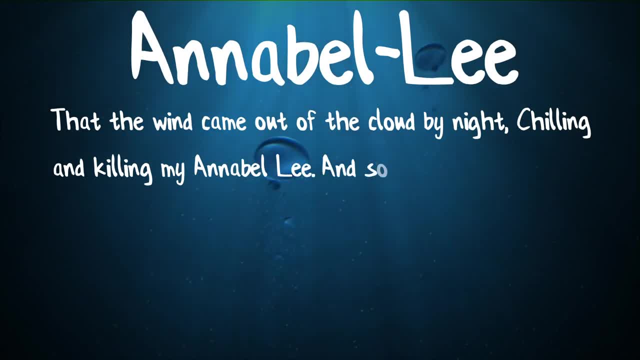 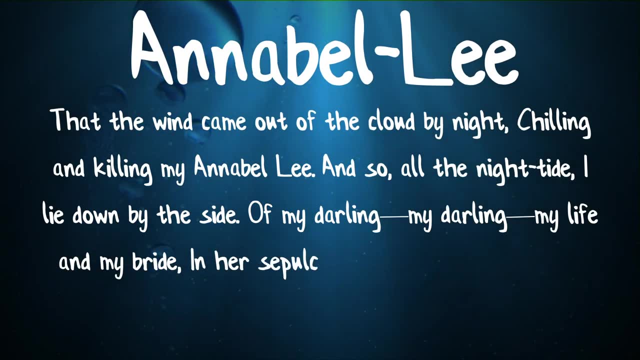 Chilling and killing my Annabelle Lee, And so all the night tide. I lie down by the side Of my darling, My darling, My life and my bride In her sepulcher there by the sea, In her tomb, by the sounding sea. 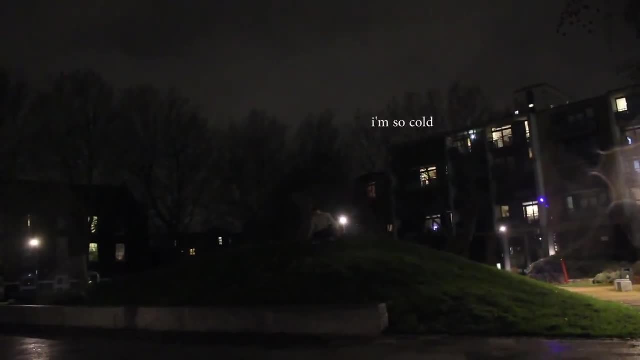 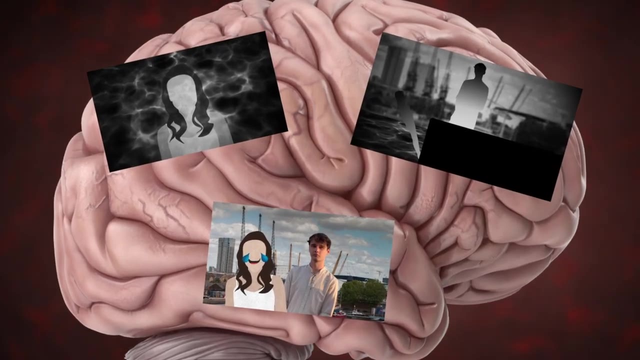 All of this would also explain why Wilbur keeps saying I'm so cold. This is the first time this event has been burned into his mind. those last words, the embarrassing moment, he himself being cold from the water, A traumatic moment so strong that it causes a mental break. 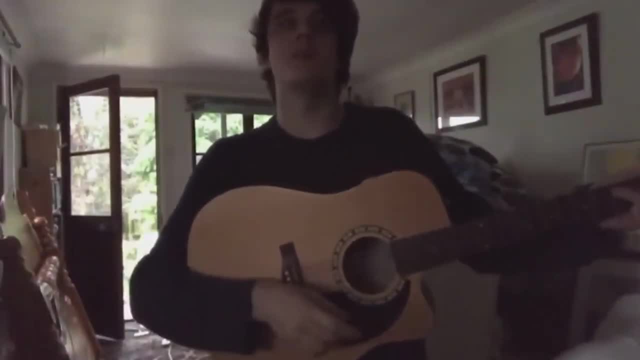 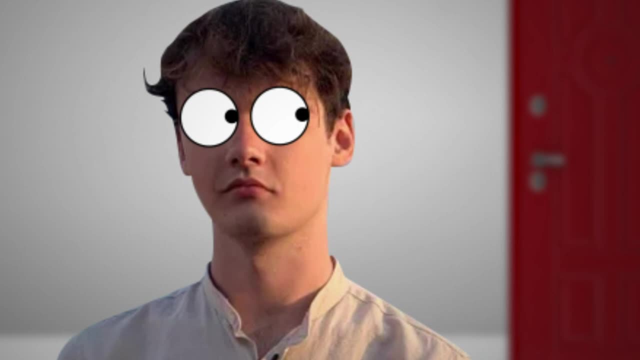 It's also a moment that would force him into hiding, explaining the knocking on his door in the first video He's running from the law, or at least it feels like he's running from it. He's actually running from a guilty conscience. 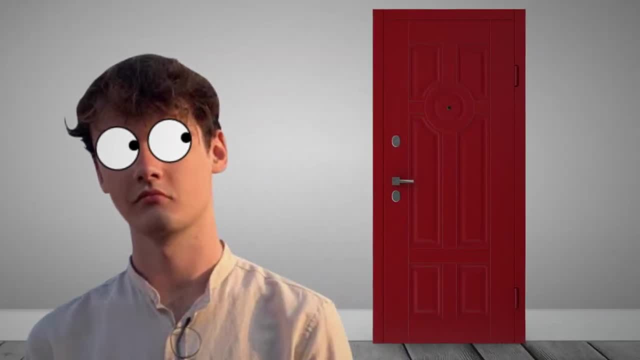 kind of like Poe's telltale heart. So any sort of knocking on the door could be the police or you know- just a threat, And so he panics and leaves every time. However, there is one small snag in this whole plan. 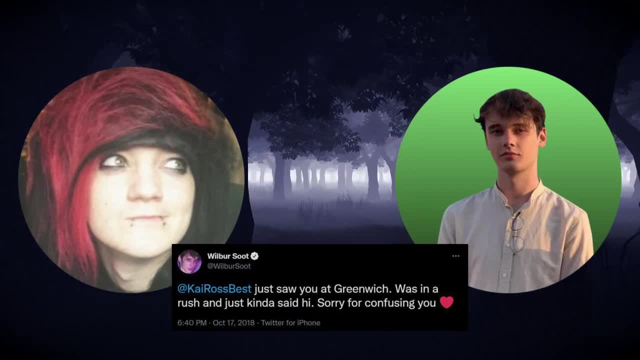 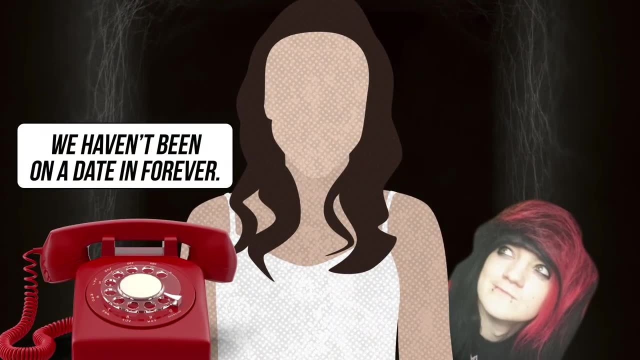 Kai. Kai knows about Wilbur After all. we know that they met in October that year, which is also probably when he met that mystery girl. She does say that they haven't been on a date in forever, So Kai knows this girl. 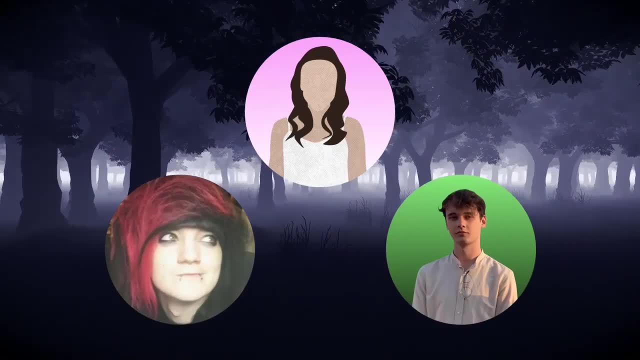 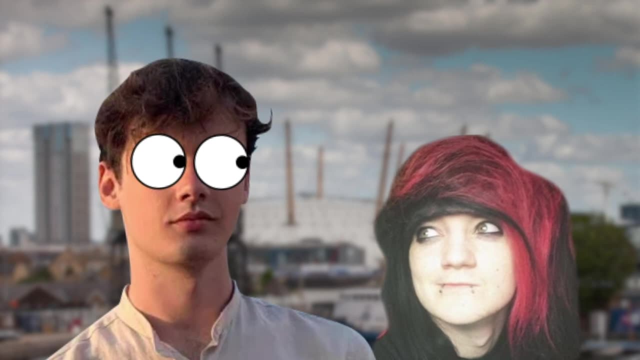 Maybe he was even in the prank that they were pulling, And so he knows that she's now missing. When Wilbur suddenly realizes this, he plots to have him removed from his point of influence as Jack's editor, Paranoid that this information will get out. 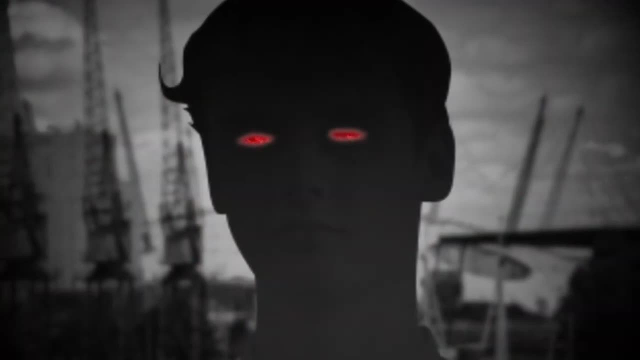 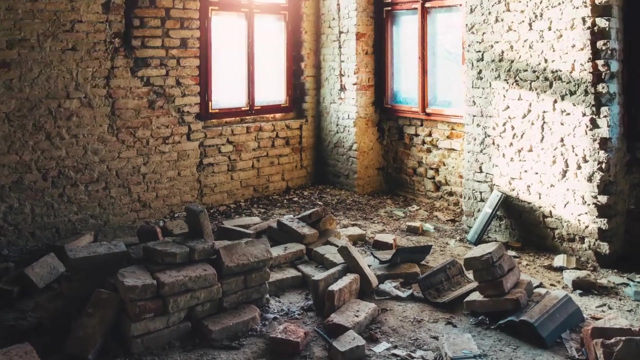 When Jack doesn't immediately fire Kai, Wilbur takes it upon himself to remove him the only way he knows, by throwing Kai into the same part of the Thames. However, Kai is a strong swimmer. Wilbur knowing that he can't get rid of Kai, 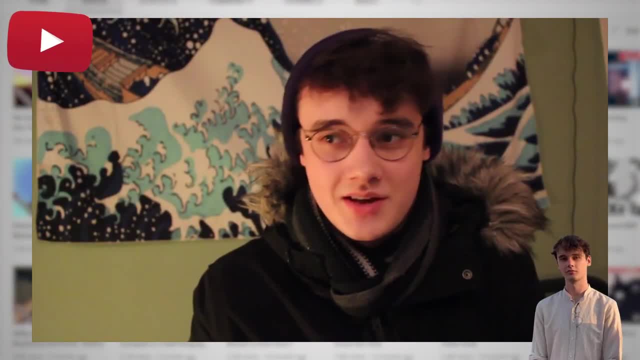 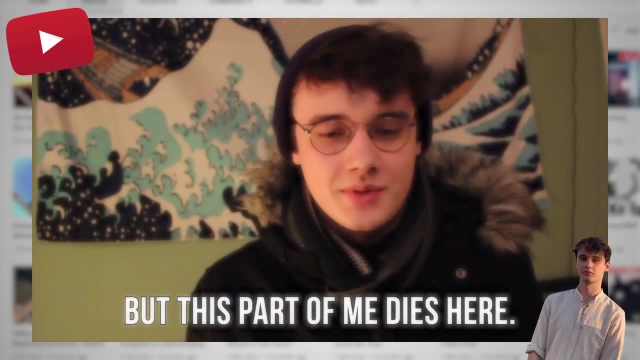 is now forced to face his actions. In his last video of the ARG, Wilbur talks about how, even though the part of him that people know will be dead, he'll still be here. This is where I die, I'll still be here. 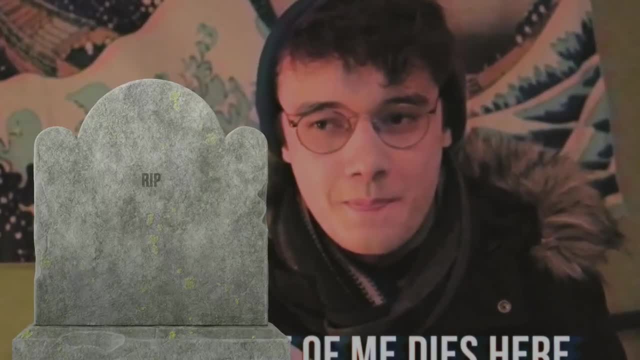 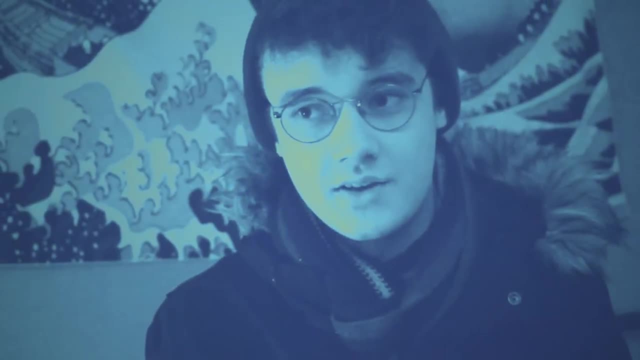 This part of me dies here, And the part of him that will now be dead is, of course, R Fakir, Who now no longer has a place in this world. as Wilbur accepts what he did, And so as he begins to explain the story to us, 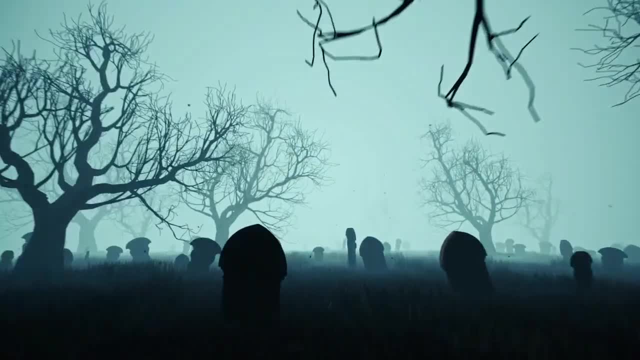 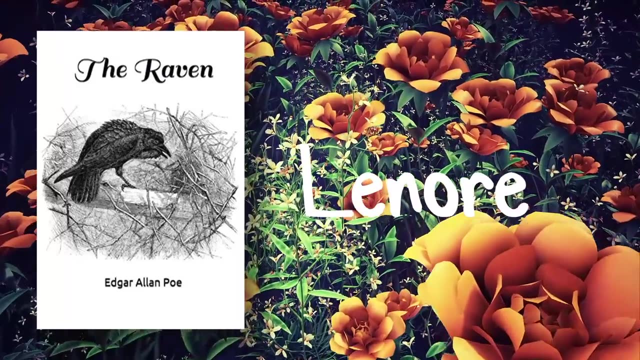 R Fakir disappears. And to round it all up, I present to you the last Edgar Allan Poe poem, Lenore, A poem about not mourning for the dead, but instead coming to terms with death and celebrating the life that once was. 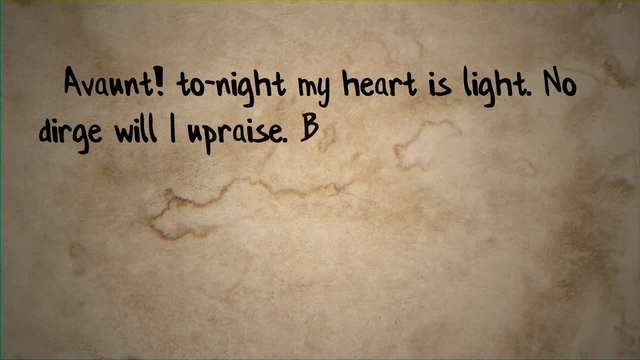 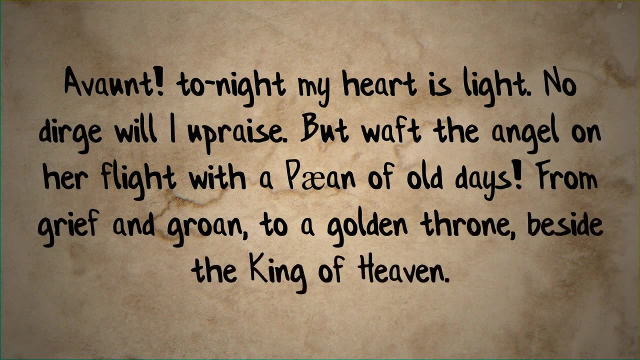 Avant. Tonight my heart is light. No dirge will I upraise, But waft the angel on her flight With a pain of old days From grief and groan To a golden throne Beside the king of heaven. All of this would make sense as Wilbur is coming to terms. 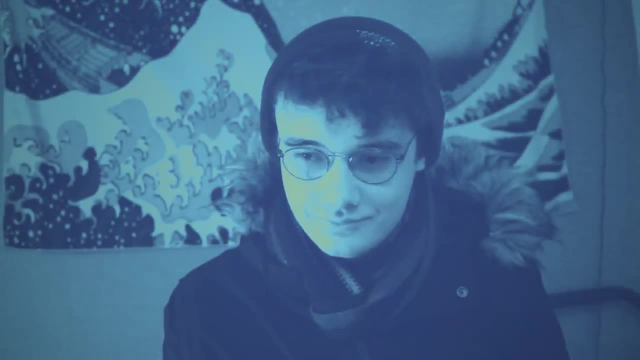 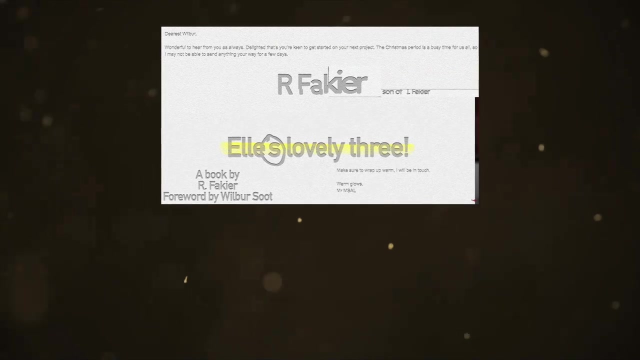 not only with the death of the mystery girl, but also with the death of a part of himself. Plus, it allows us to solve the mystery about why R Fakir's book is called Elle's Lovely Three- All three of the poems I've mentioned.